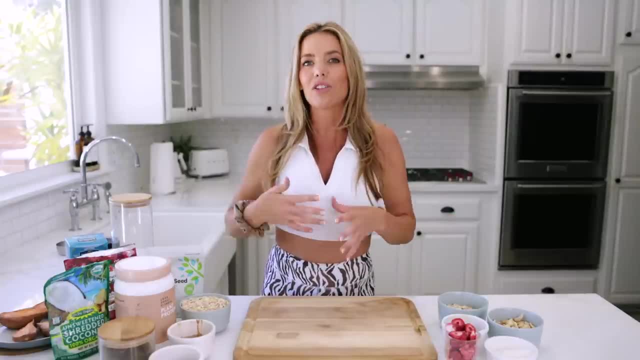 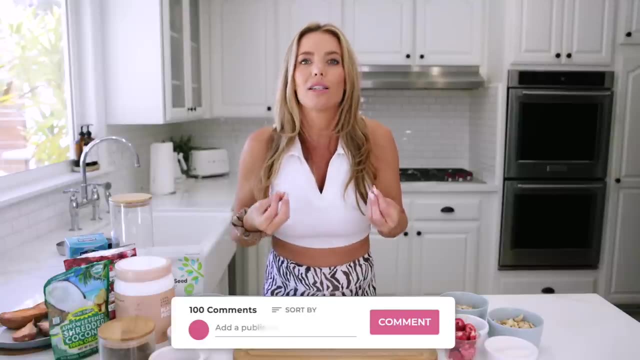 snacks And then if you guys like this idea of like a series, then maybe I'll start doing like snacks lunches. So if you do hit the thumbs up and comment down below and let me know like which things you want to learn to meal prep better, just to make your life easier. One thing I love: 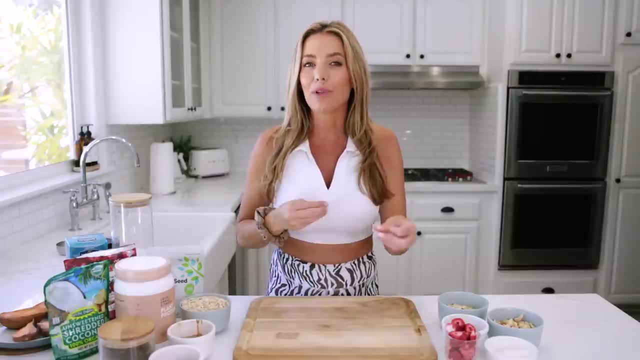 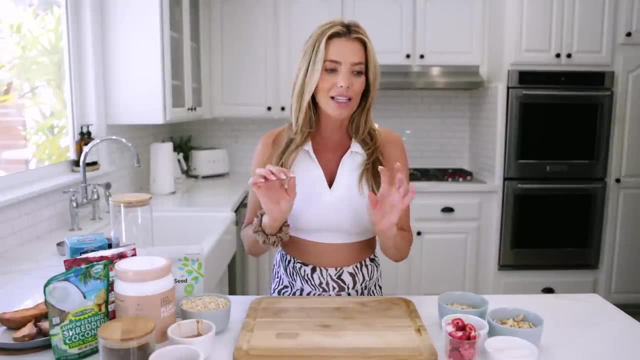 about the recipes I'm going to show you guys is a lot of them have similar ingredients, so you're not going to have to buy like a million different things to make all five of these snacks. They're simple. You can make little tweaks and swaps to make them your own, but they're so delicious- a little summer inspired. 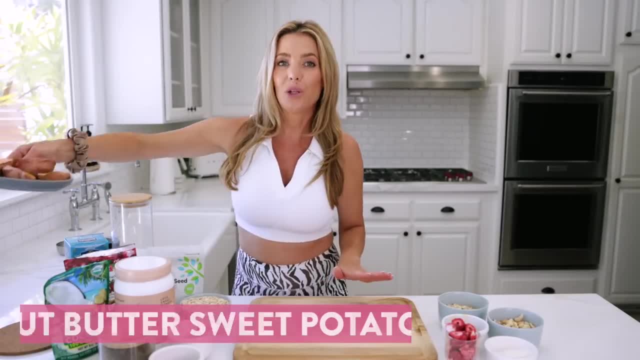 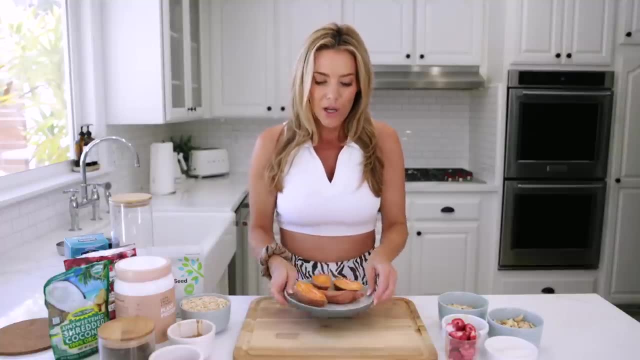 and I know you guys are going to love them. So this first snack is a really good one, especially like either before or after a workout, to help fuel your body with those healthy carbs. So carbs are important, We know this, but sweet potatoes are such a great source of not only healthy, 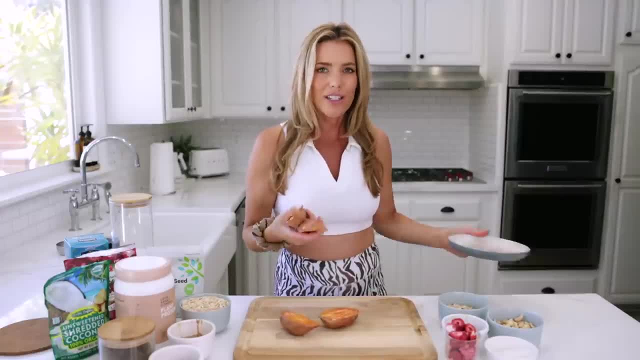 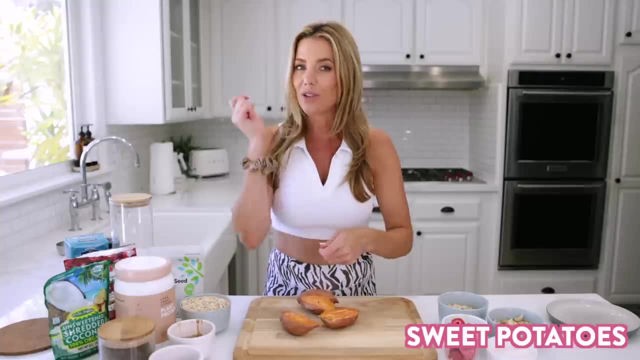 carbohydrates, but also a lot of fiber. So I just cooked these up in the microwave. You can cook them however you want, but again, I'm all about making things easy. So I had two small sweet potatoes, cut them in half, put them in the microwave for five minutes. 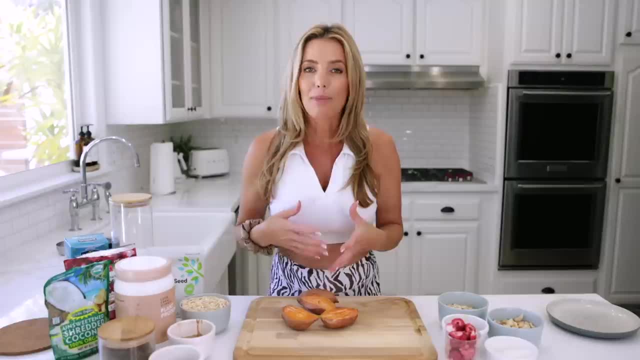 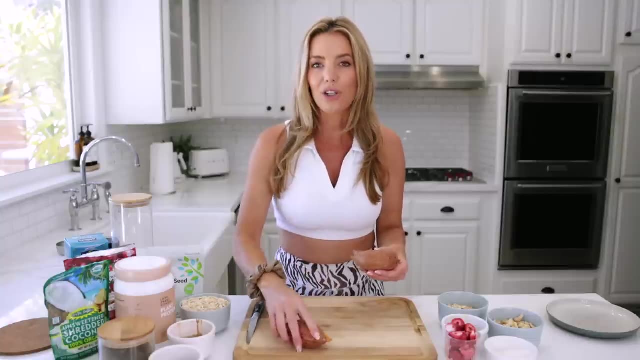 They're cooked all the way through, And this, again, is something you can prep. So I'll put these in containers and store them once they're ready. So let me show you what I do with them. You'll notice I have different size sweet potatoes, So I will usually eat the smaller one. I'll give Ryan the. 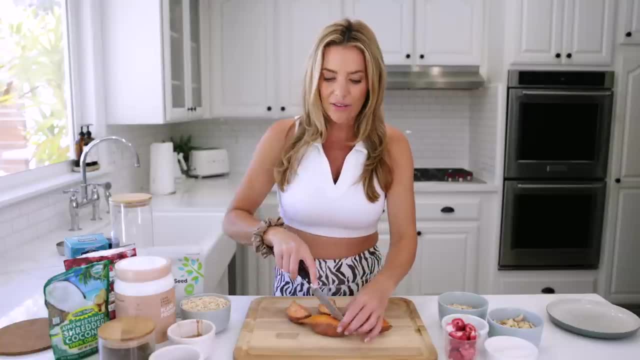 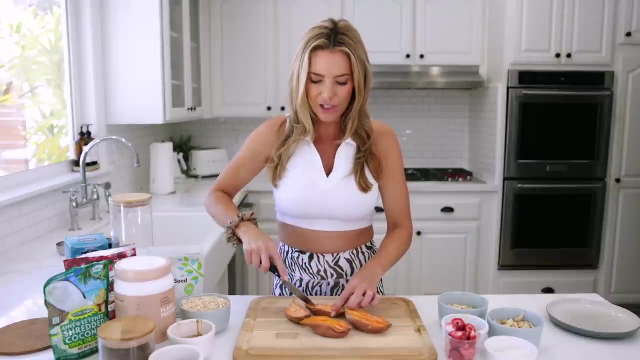 bigger one. So if you're meal prepping for like a family, you can kind of do it that way as well. But once they're cooked I will cut the halves in half again, not all the way through the skin, just kind of through the meat of the sweet potato. 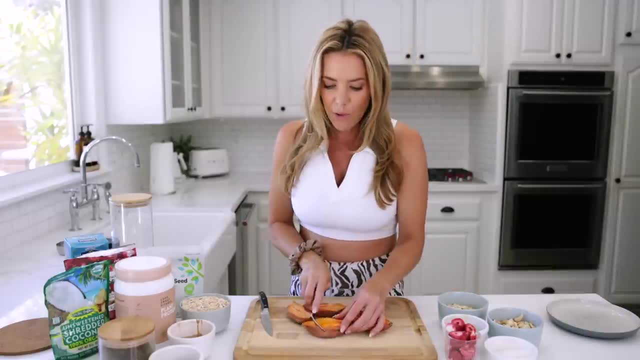 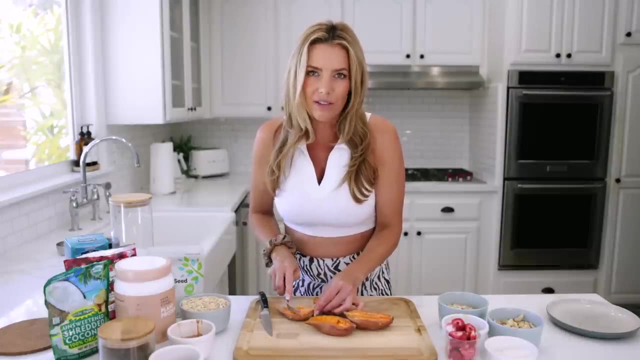 And then I'm going to take a fork and kind of just mash it a little bit. You don't need to get crazy, because we want it to stay within that skin. Think of like potato skins, right? Same kind of thing, sort of. So just give it a little bit of a mash So it opens it up a bit more. And then this: 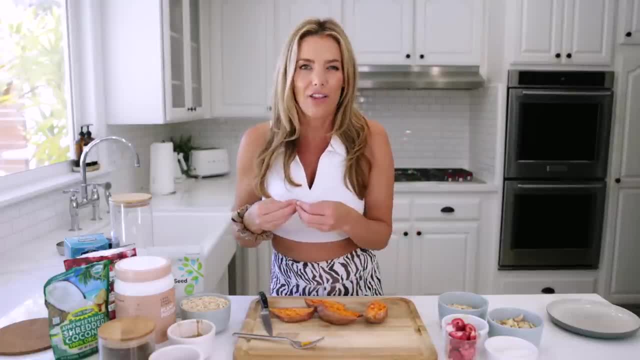 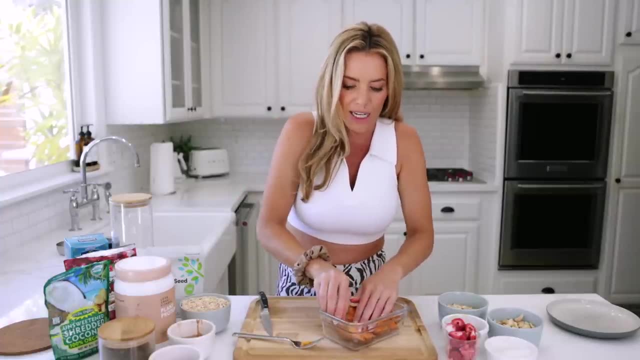 is when I'll actually put them in the containers, because it helps keep everything together a lot better. So I just have a glass container. I'm going to line these in here And, depending on your sweet potato size, you might need larger containers, but I like to do it that way. 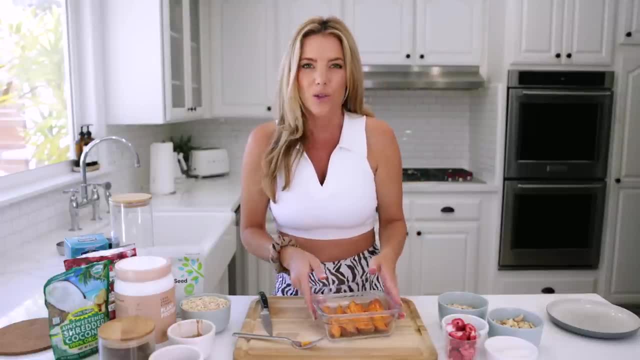 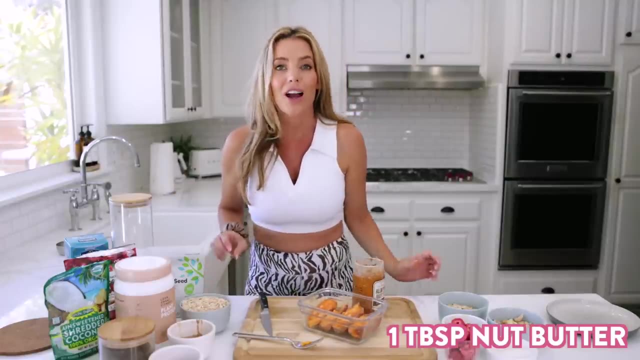 I like using these sweet potatoes are more like the size of my palm, So it's a good, healthy portion. And then, once we're in there, I'm going to take some almond butter. You can use peanut butter, You can use cashew butter, any butter you like, really doesn't matter at all, but this is. 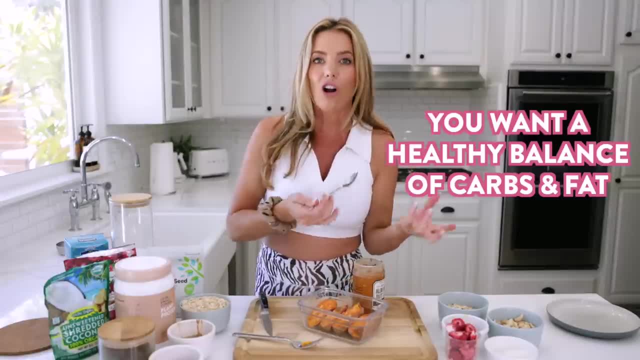 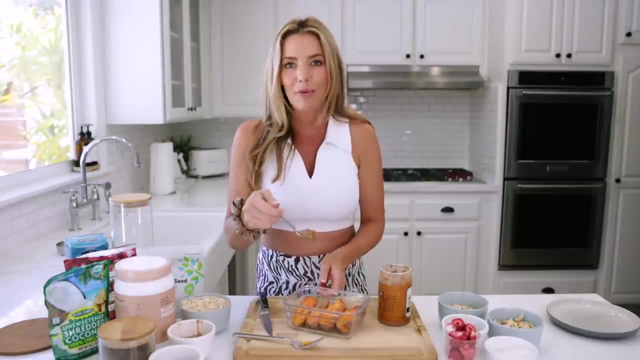 going to give you your healthy fats. You always want that balance of your carbs with your healthy fats. Um, you also get protein in your nut butter And then, depending on the texture of your nut butter, sometimes you can just drizzle it on there. Other times you kind of have to spread it. 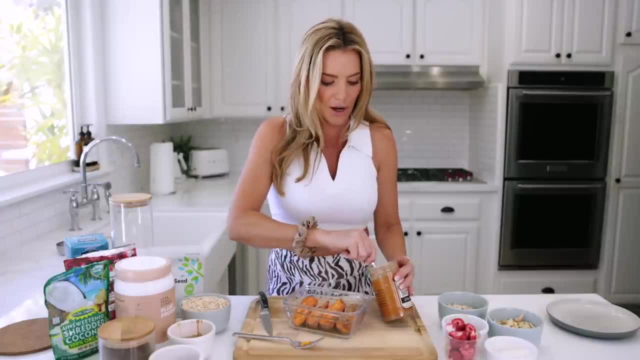 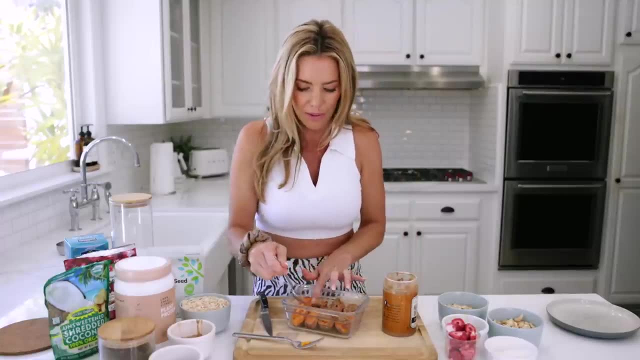 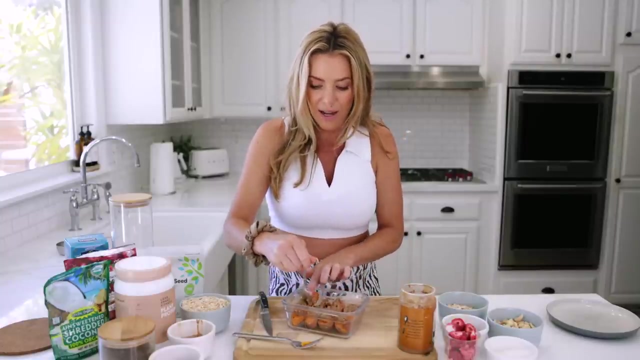 but I'm using about a tablespoon Of nut butter for each half and just spreading that right on top And like, besides the five minutes it takes to cook in the microwave, these take about two minutes to actually prep, which again makes it such a good, easy, healthy snack. And then, for the top, I like to mix things up. 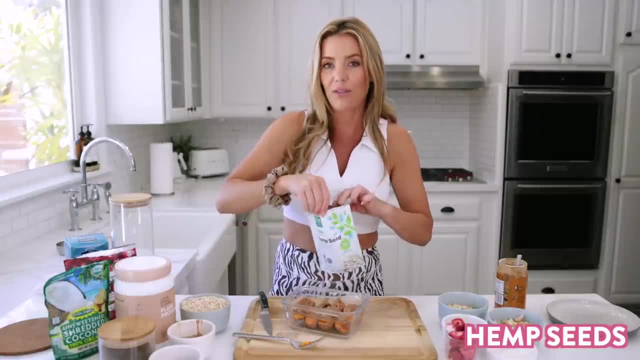 So I'm going to show you some of my favorite toppings. Hemp is really amazing source of healthy fats as well. We're just going to use a little bit of them, but they also are an incredible source of protein, which is kind of unexpected. 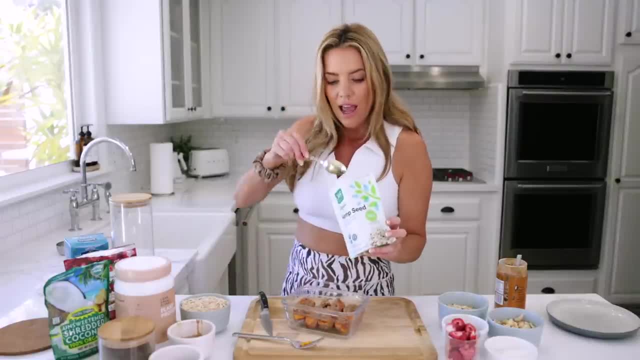 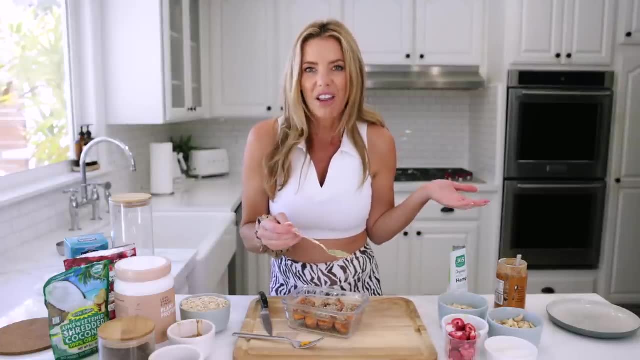 So again adding some more protein into the mix here, And then this is not anything I measure. I literally will just sprinkle it on top until it looks like good and gives it a little bit of a crunch too. So just sprinkle it right on there. And then I also like to put some unsweetened 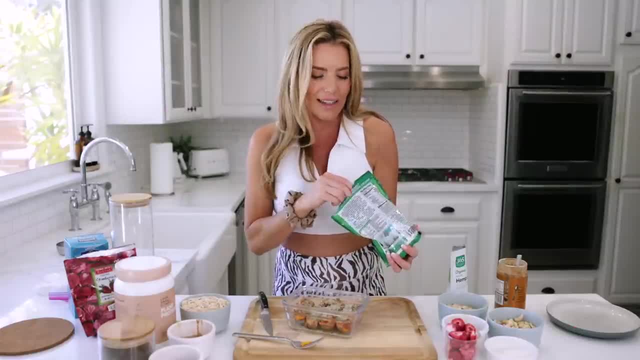 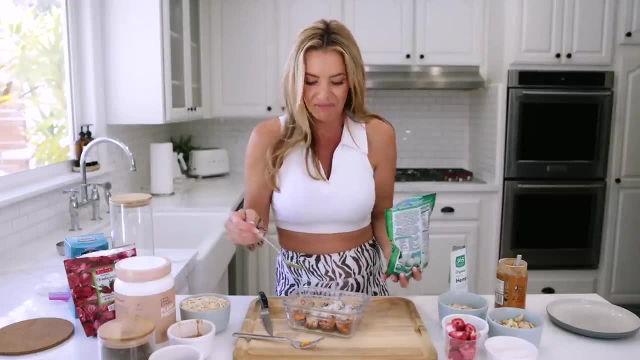 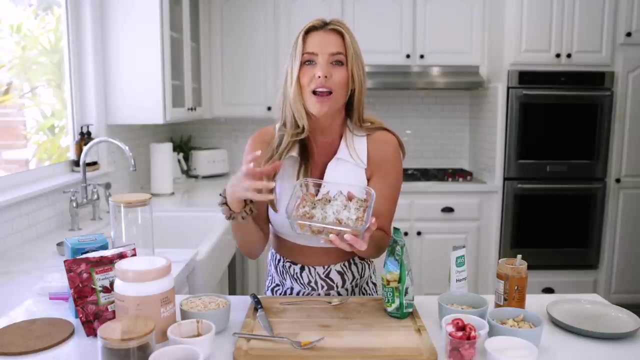 coconut flakes. This gives it such a yummy like savory sweet snack vibe. And then again, just no measurements required. Just go ham. If you love coconut, go for it. But really, like you can put chopped dates on here, You can put crunch nuts on top, whatever you want. 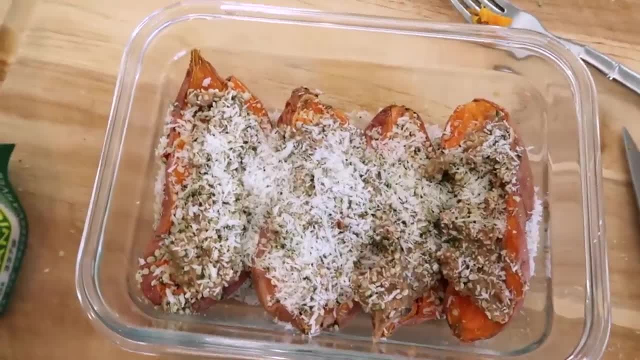 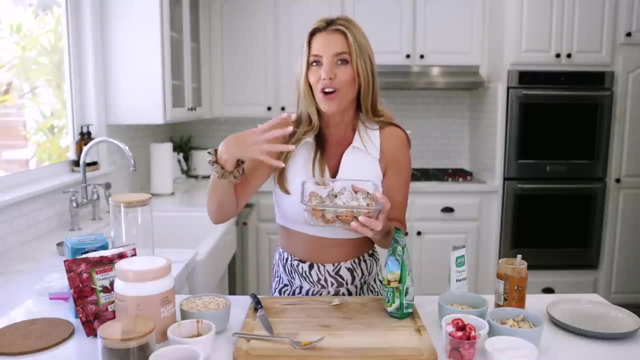 If you want more of that crunch. it makes it so delicious and allows you to mix it up more, but you're getting everything you need in that snack to help kind of keep you full and also make sure that you're getting all of that fuel. I just realized that my hair is down and I know I'm going. 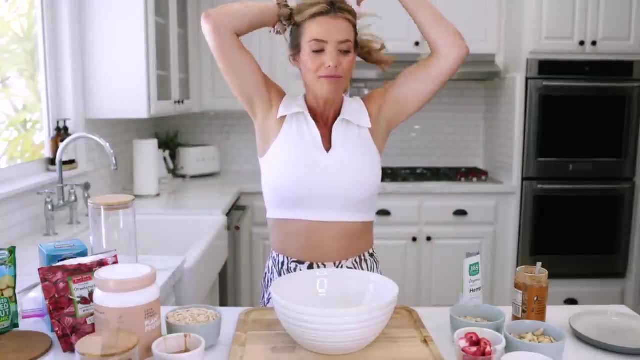 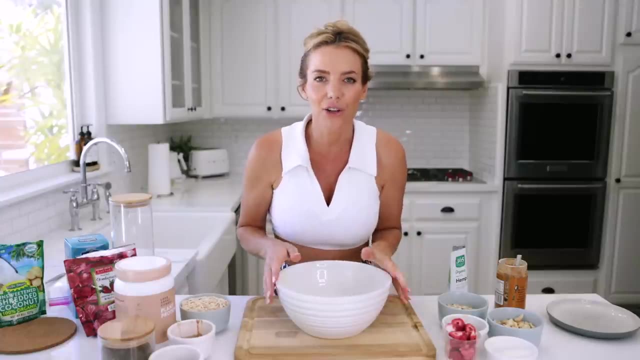 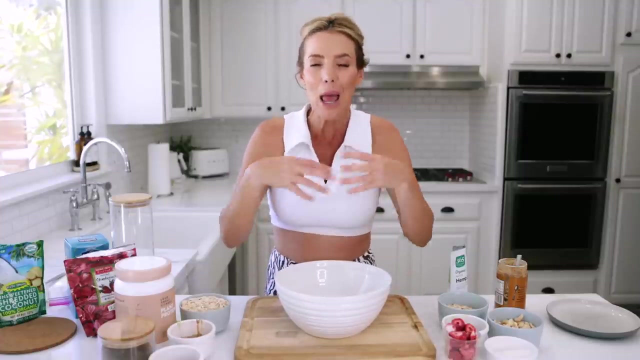 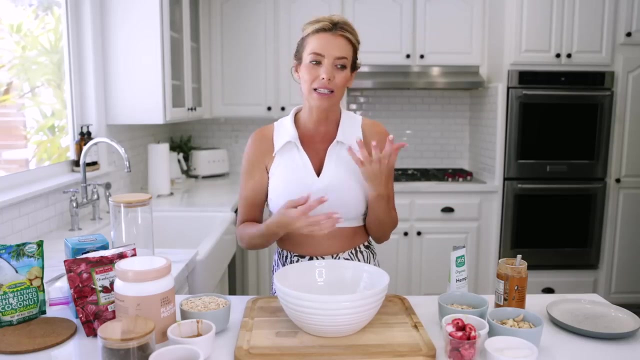 to regret it later when I find that like piece of hair in my snacks. So, as always, try to put your hair up when you cook, Okay. So the next snack I have for you is actually like you can just snack on it by itself, but it's one that you can use in a lot of different ways, which again makes it a really good one to meal prep for the week or weekend, so that you have that like versatility. So this is actually a delicious peanut butter protein granola. I've been making granola forever. I usually keep it kind of simple. I'll mix up the nuts and things I'm putting in it, but I wanted to make this one packed with protein because you're getting the healthy carbs already in the oats. 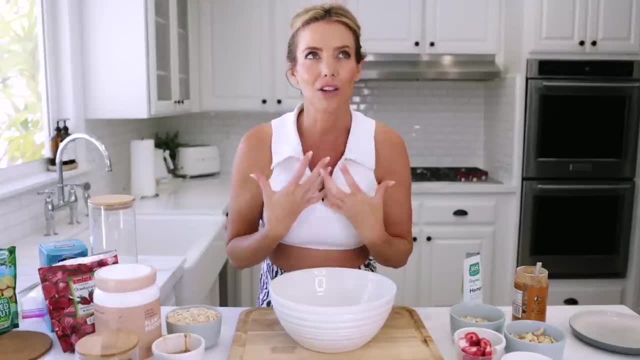 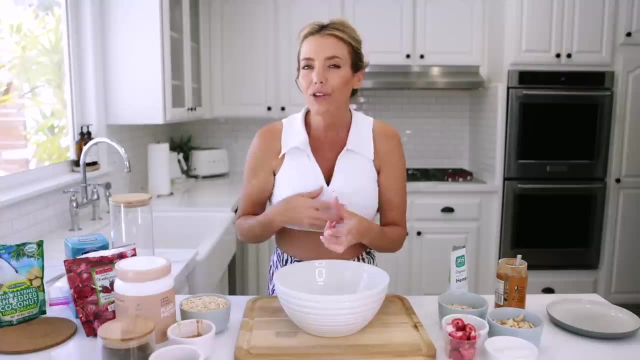 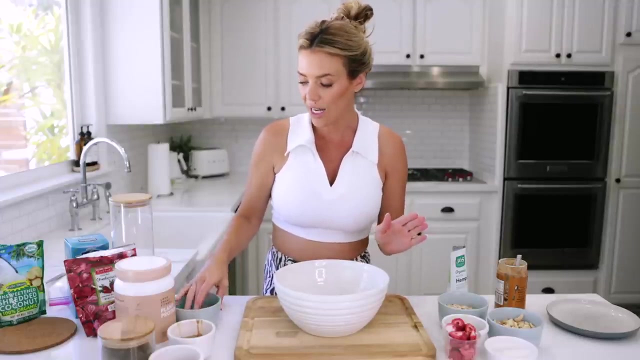 So I'm just going to cover all of those nuts and things. Get your you know the kind of stuff that you want to put in there, but also give it that yummy peanut butter flavor. I'm a huge peanut butter fan And I feel like it just makes it easy to throw on top of yogurt If you're having like any type of like fruit or nuts and you want to have that mixed in there or just again add more nuts to it and have it be just a snack you have on the go. I'm going to start with two cups of oats, So just put those right in there. These are gluten-free rolled oats. You can really use any kind. I think these are Bob's Red Mill. You guys always ask the brand. I'm not usually particular about what they're called. I'm just gonna like use the original brand for free, But these are the kind that I really like to have on top of yogurt, Like I would be using a lot of other nuts in here. I'm going to add a little bit of. 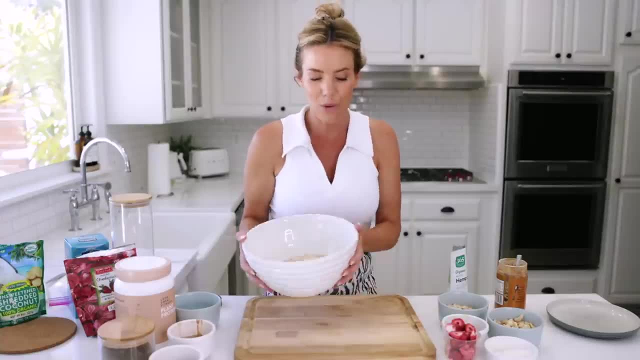 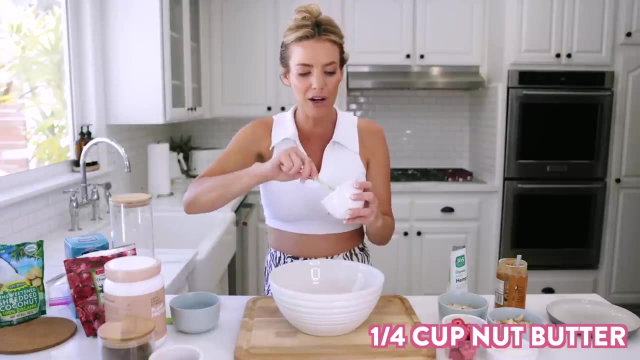 my hands with stuff. as long as it's like organic, gluten-free, that's what i go after, but two cups of any type of rolled oats. you want to start it out, and then i'm gonna use a quarter cup of peanut butter. this is crunchy peanut butter. you can use whatever you want. i just love crunchy peanut. 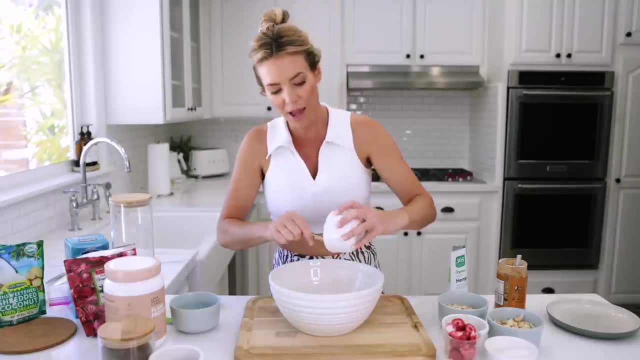 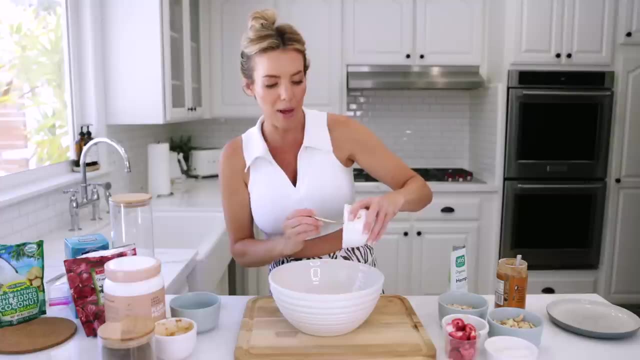 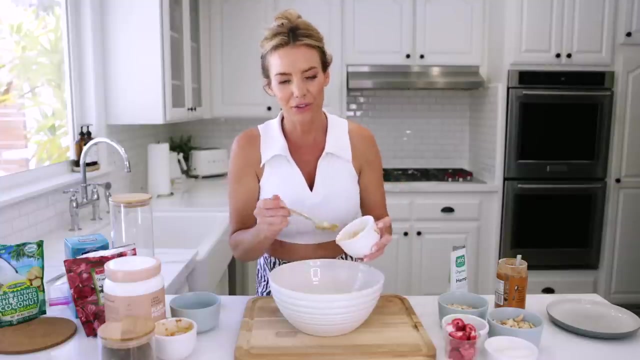 butter again. it just adds more texture. so i'm just gonna drop that right in the bowl and i also have a quarter cup of maple syrup. you can also use honey for this, but i really like maple syrup just because it's like lower in the glycemic index and it's nice and flavorful. this is optional. 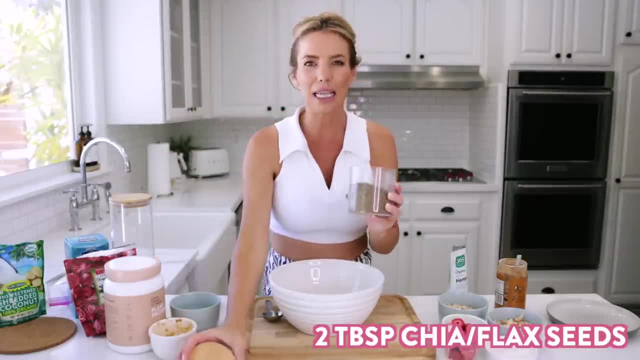 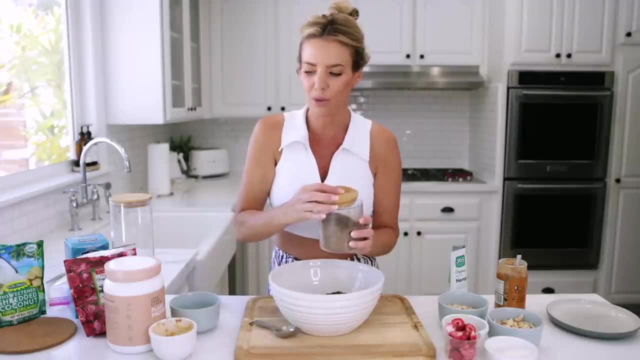 but i have a combination of flax and chia seeds that i always keep for, like smoothies and things, so i'm going to put about two tablespoons of that combination in there. you can do one or the other as well, and it'll also help bind everything together. and then, last, i'm going to add the. 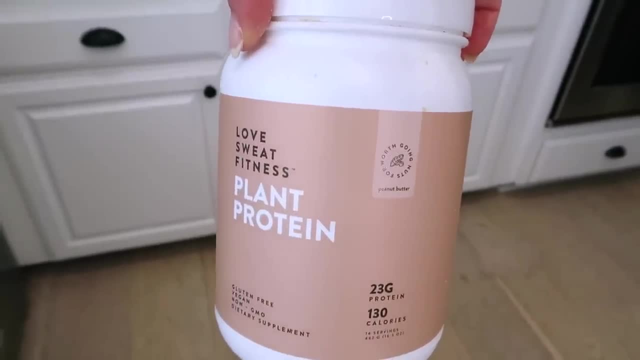 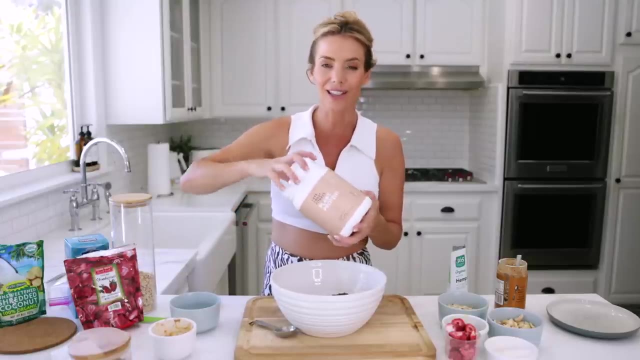 love soap and this plant protein and the peanut butter flavor. if you guys haven't tried this one, it's everyone's favorite right now. like people are obsessed with it, i get it. it is so freaking delicious and it has 23 grams of protein per scoop and zero grams of sugar. 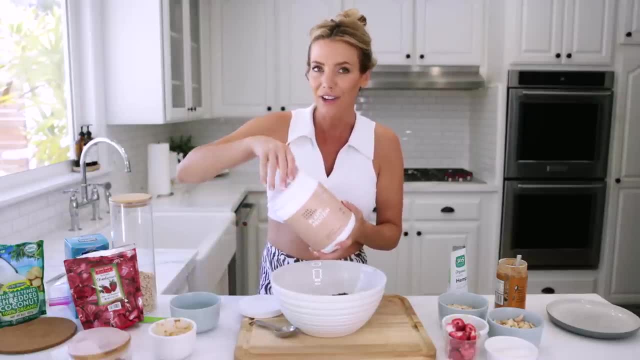 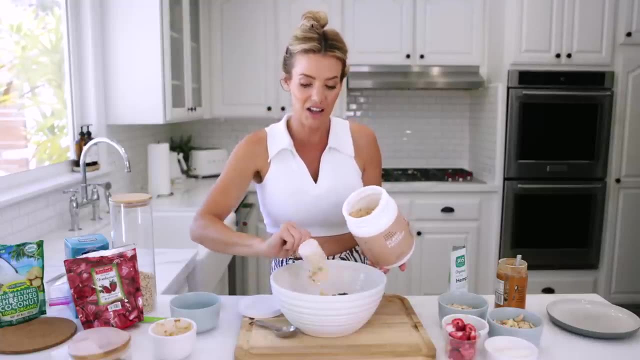 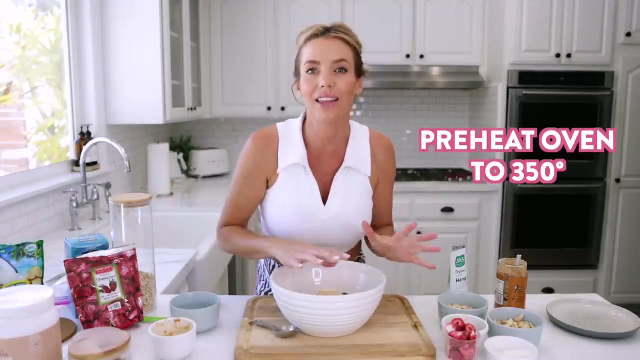 vegan, gluten-free, dairy-free, soy-free, everything you want, and a protein powder. so for this i'm going to actually do two scoops as well, so getting 46 grams of protein right there, and i forgot to mention this. but you'll want to preheat the oven to 350 because we are going to cook this in the 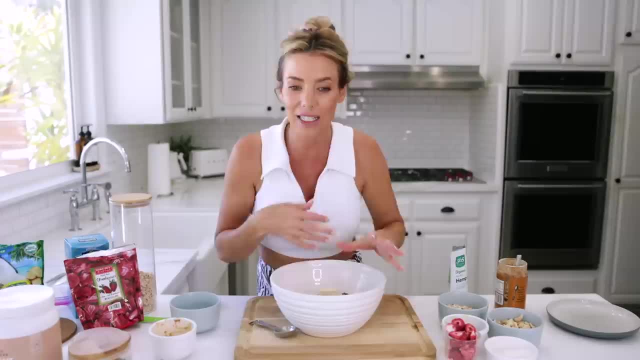 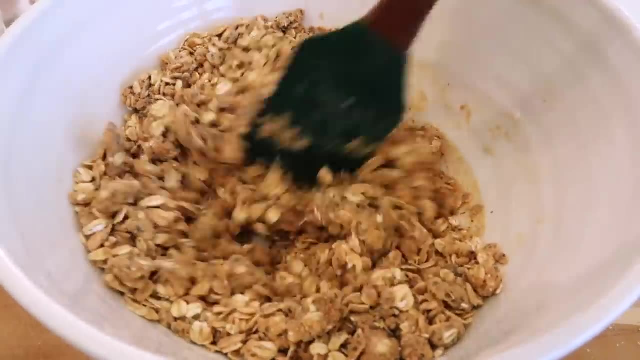 oven. so this is another one. it takes about three to five minutes to prep everything, and then i'm going to put this in the oven for about three to five minutes, so when you're done with everything, then you just stick in the oven and you don't have to think about it once everything is in the bowl. 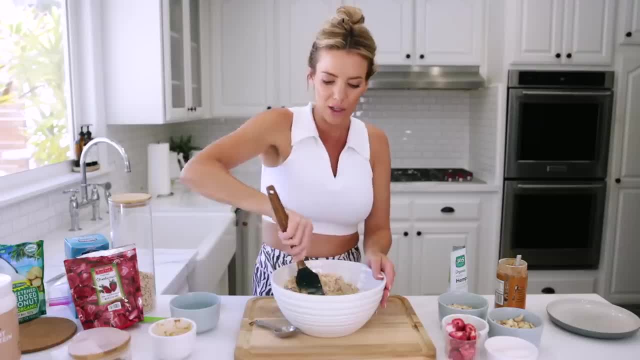 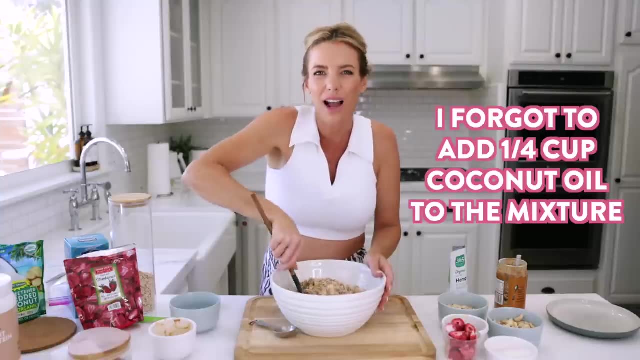 you're just going to mix it all together and you can kind of eyeball this if you get it mixed up and you're like, oh, it needs a little bit more oats, or i want to add a little bit more peanut butter, depending on the texture you're going for, but you want to get it. so it's kind of like not. 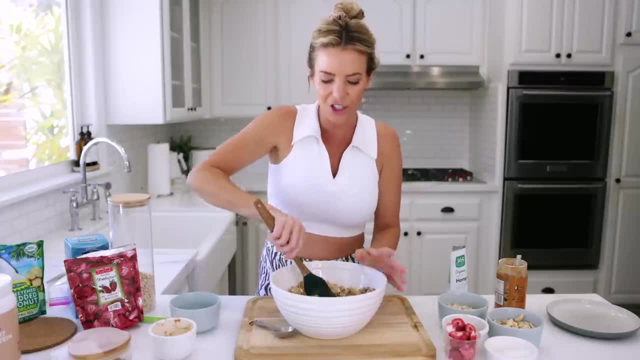 quite a dough but, um, getting close to a dough. okay. so once you get that texture, you're going to notice there's some clumps in there from the peanut butter. that's totally okay. they're going to melt down a bit and then i'm going to add that back in the oven for about 30 minutes and then i'm going to 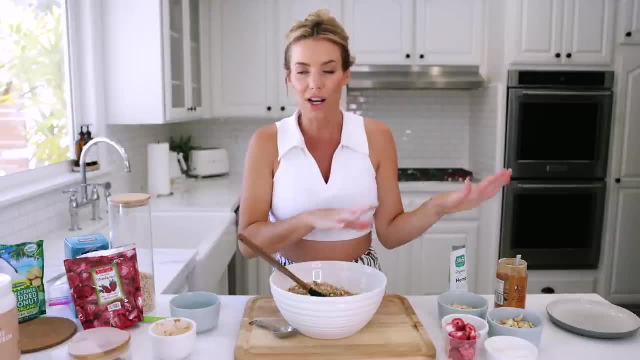 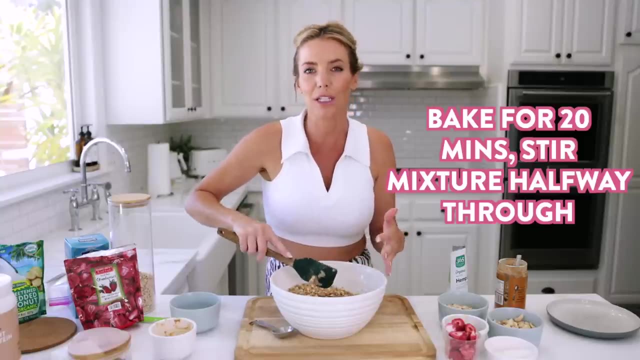 then I'll show you like, basically what we'll do is, once the oven is ready at 350, you're going to put this in for 10 minutes. it'll start to kind of form together most of the time. so then you'll just kind of use your spatula or something to break it up a bit again and mix it up and then cook it for. 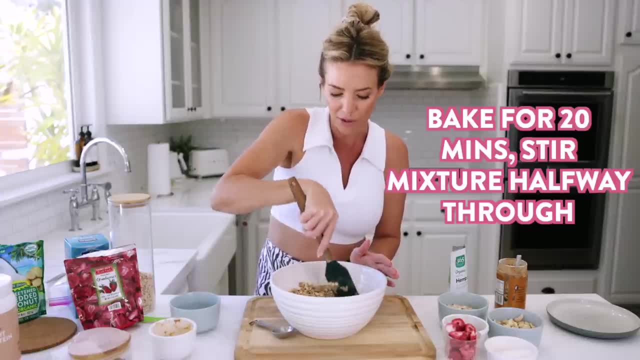 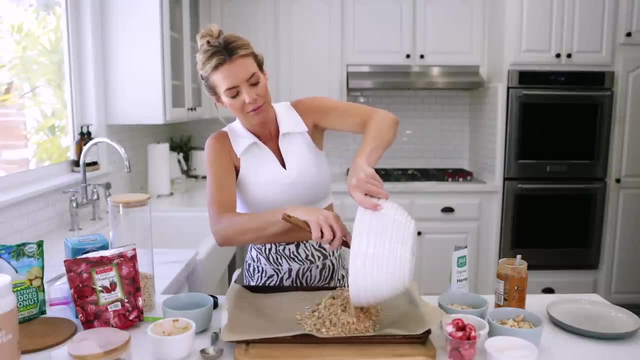 another about 10 minutes until the oats get a little golden brown. I have a sheet, just a baking sheet, lined with parchment paper, so we're gonna just put this right on there, and then my hands are clean, so I'm just gonna use my hands to kind of press it in a bit and maybe break up some of 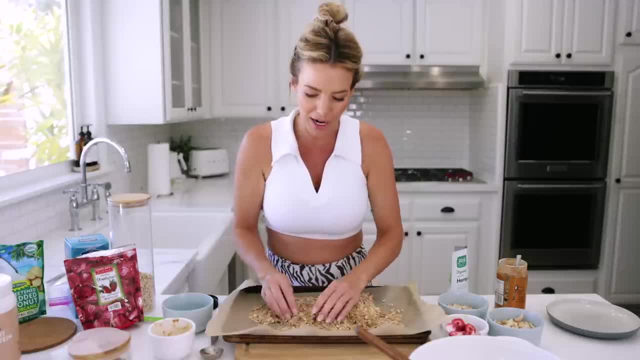 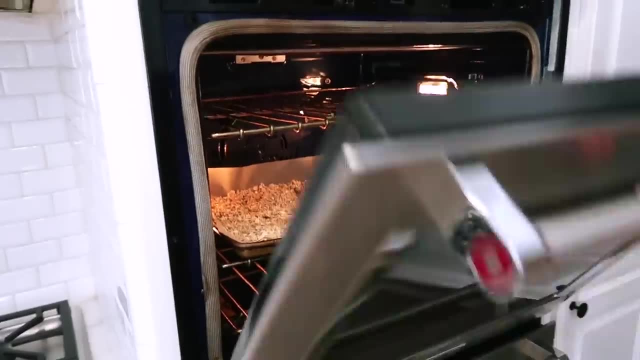 that peanut butter just a little bit more, and you can do that so much better with your hands. so if you don't mind getting a little messy, just do that and then just spread it evenly on the parchment paper and stick it in the oven. the last two snacks I've showed you guys are more on the sweet side. 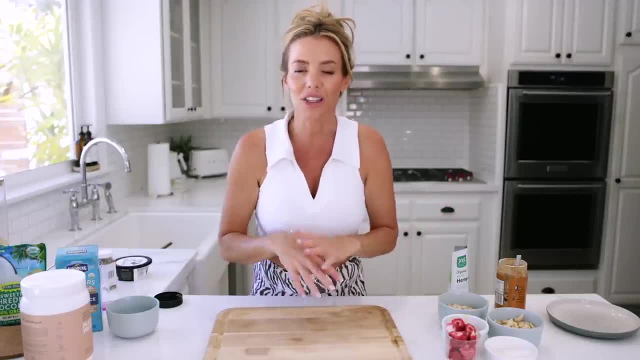 like the sweet potato. one's like a little savory but more on the sweet side, so I want to show you one that's a really easy savory snack that I think you guys are gonna love. I've been doing a lot with rice cakes. I've always loved rice cakes. I've always loved rice cakes. I've always loved rice cakes. 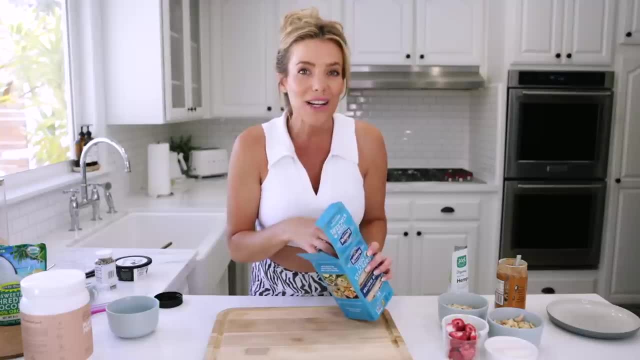 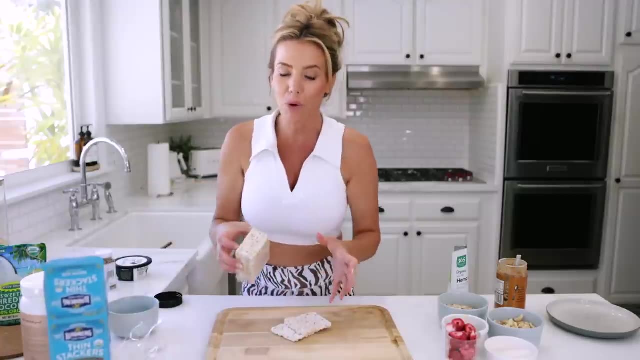 if you guys have used my meal plans before, you see, there's rice cakes in there all the time and I like to mix up how I make them, but this is one that's again a really great go-to to be able to prep, or if you just need to make a snack really quickly, I've got you the great thing about using. 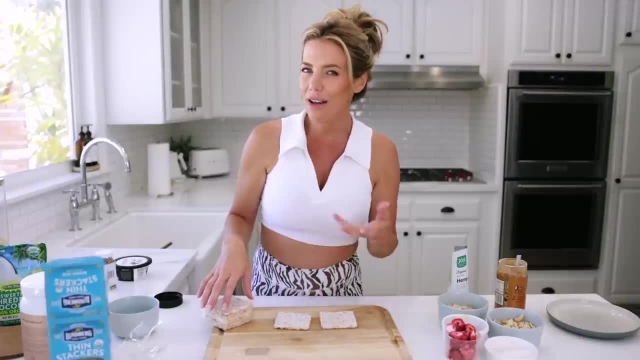 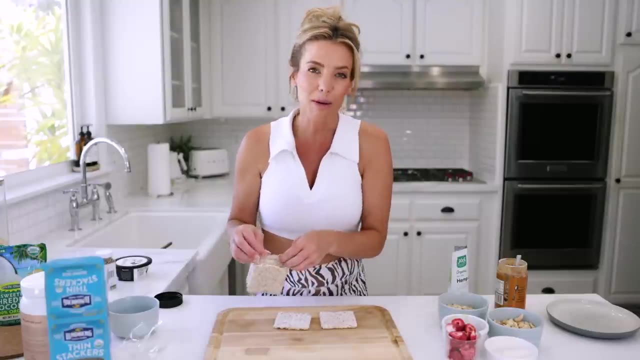 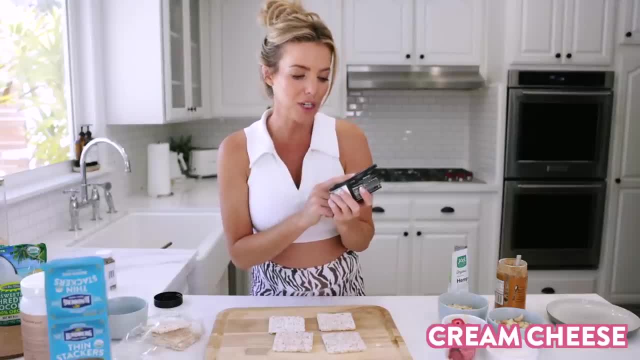 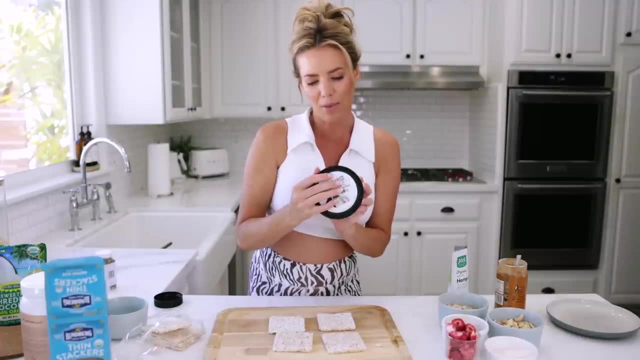 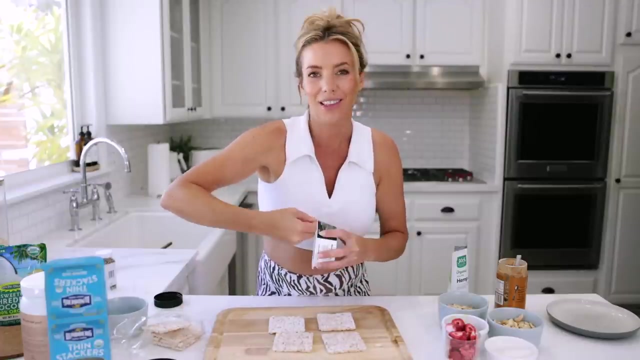 however you want. I'm using this kite hill cream cheese. this is a like everything. like an everything bagel seasoned. it's a non-dairy cream cheese. I think it's made with almonds, yeah, um, but you can use regular cream cheese if you want and then obviously like any flavor, but I just love. 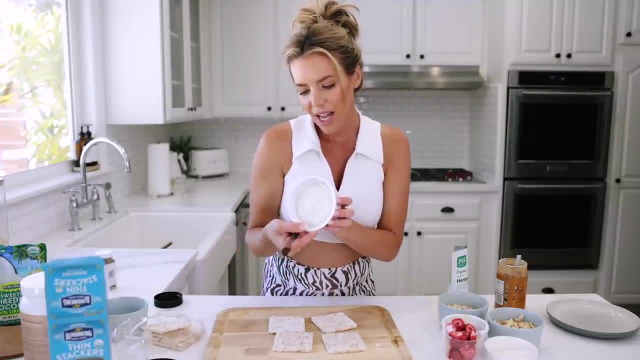 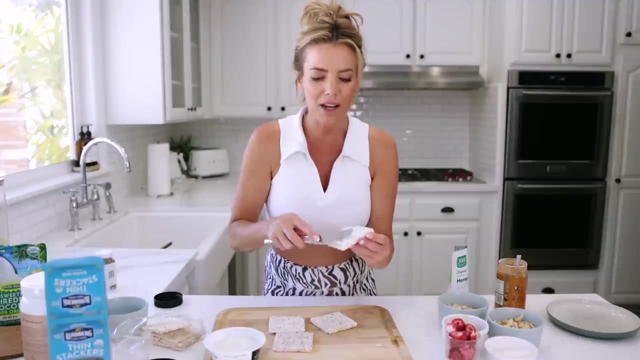 everything bagel flavor. so we're gonna open that up. and then serving size: what is it? two tablespoons, so I'll probably put about a tablespoon on each one, but I'll spread it thin. so maybe not quite a whole tablespoon, but I'll spread it thin. so maybe not quite a whole tablespoon, so I'll spread it. 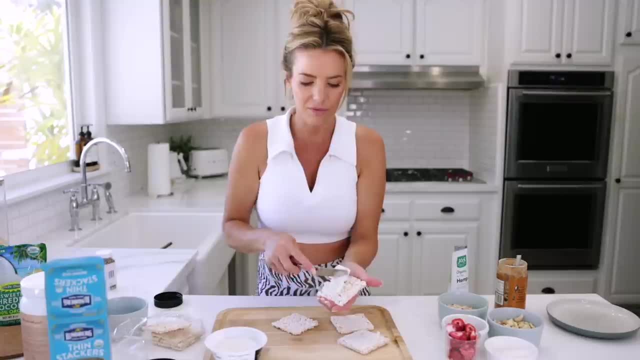 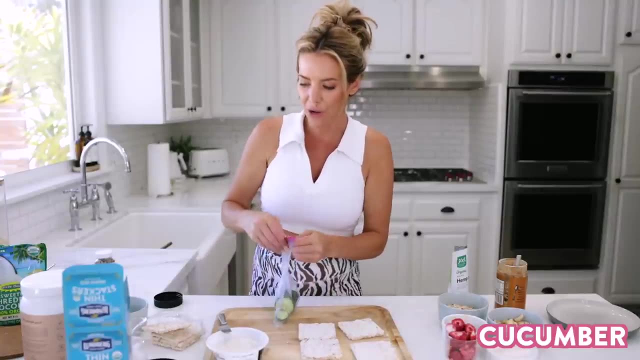 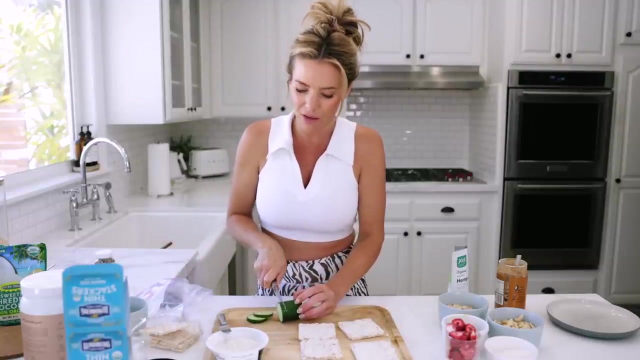 like more, like a half a tablespoon. share the love. and these are just lightly salted brown rice rice cake thins and I'm gonna take some fresh cucumber and slice that up- just really thin slices though, like if it's too thick it just makes the texture really weird. you guys see how thin these are like. 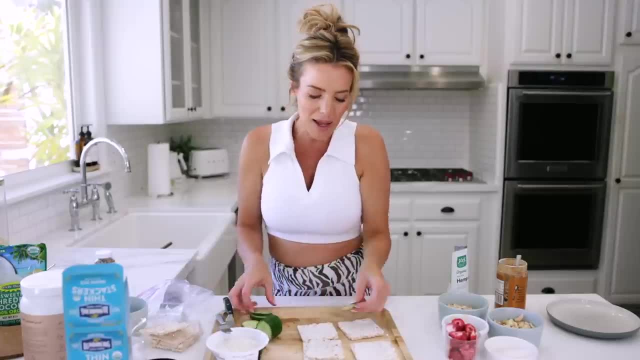 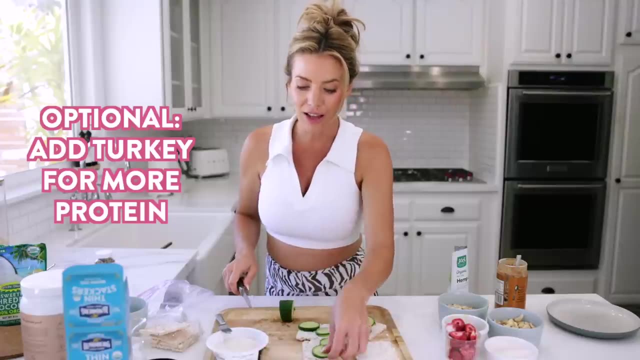 think like thin, like you're gonna put them on your eyes and then, depending on how many you want, like usually two or three on each one. this is also good for like a little bit of a cake, but I'm gonna also good if you wanted to add like turkey and actually add some more protein to it, it could be. 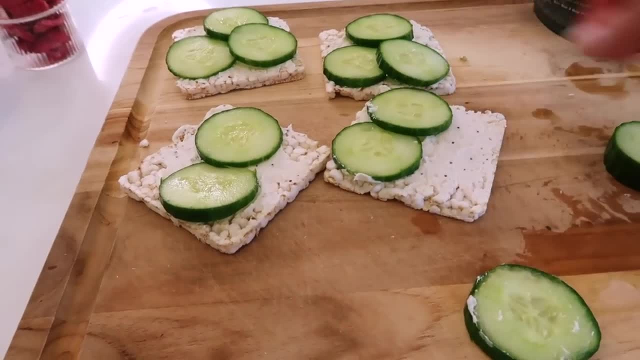 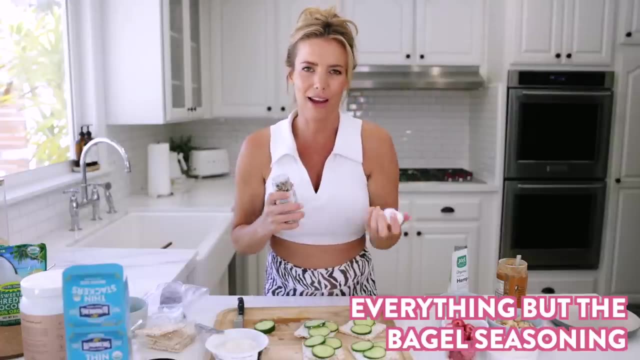 a lunch, but still could totally be a snack too. but some just like deli turkey meat would be really good on this too. and then I'm gonna use this everything but the bagel seasonings from Trader Joe's- I think everyone, like every grocery store, has it now. but again, if you're like, oh, I want. 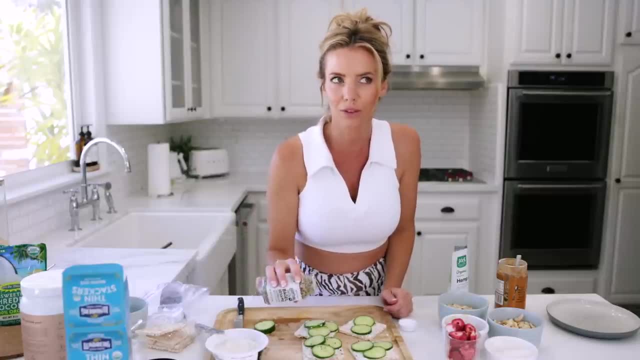 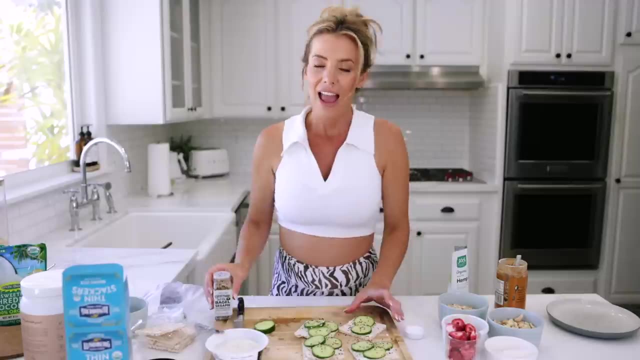 some garlic or paprika or like some hot sauce. should I put hot sauce? oh yeah, let's try that. okay, then I'll just sprinkle it right in and then I'm gonna put it on my plate and then I'm gonna put it on top. and here's the thing: if you leave them plain like this, or even if you're a turkey- 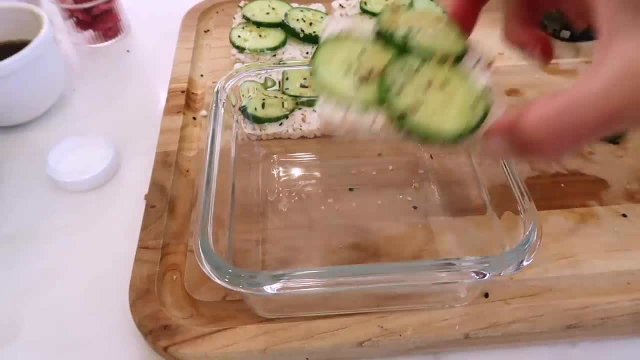 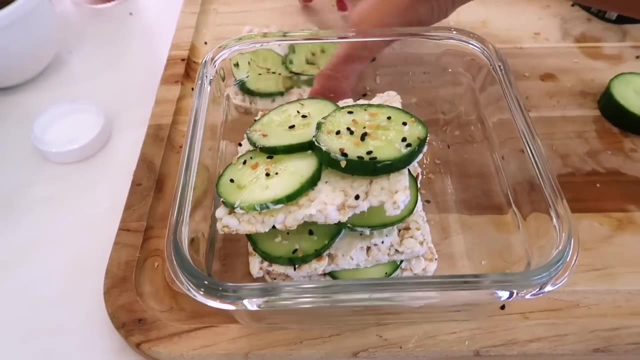 on them. it's really easy because you can just stack them and they're not gonna get like soggy. the cucumber and stuff helps separate it. that's not just like saucy. so if you do want to add hot sauce, just wait until you're actually gonna go eat them to add the hot sauce. but otherwise I 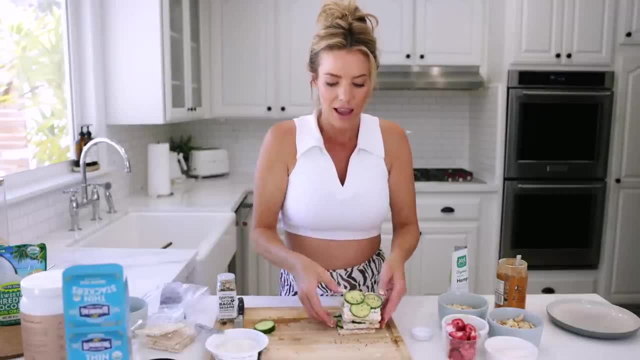 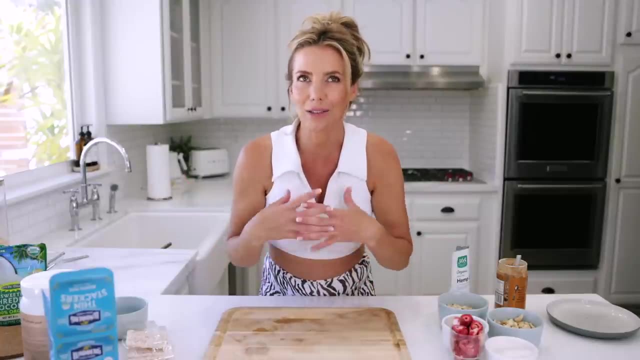 like to just stack them up like this and put them right in a Tupperware glass container and you're good to go. I told you guys like to do a lot with rice cakes. just put them in a Tupperware glass container just because they're so versatile. so we're gonna hit another one, but this one is gonna. 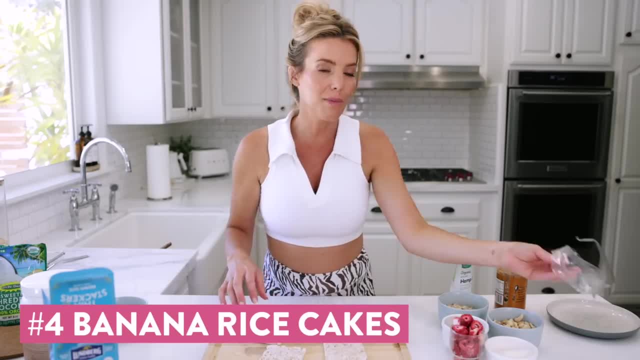 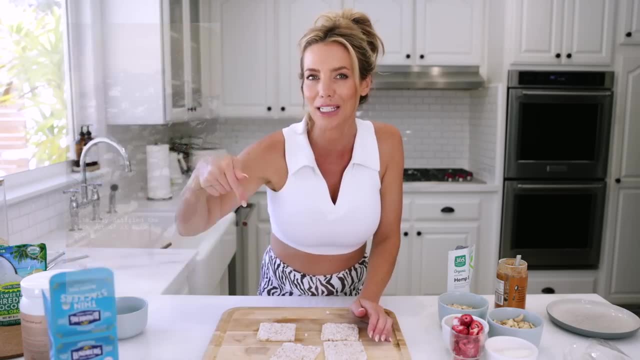 be a sweet one. I don't know if you saw my Tik Tok or Instagram. I made something similar to this, but made it like a dessert edition with chocolate and everything. if you haven't seen it, I'll link it down below. definitely go do it, because you're gonna want to make them, but this 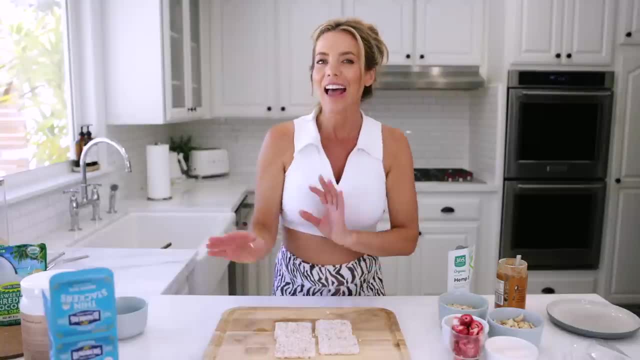 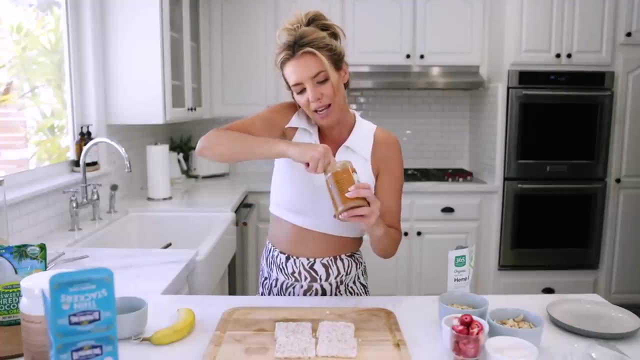 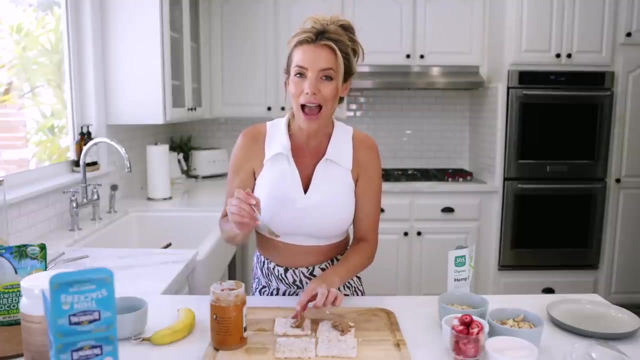 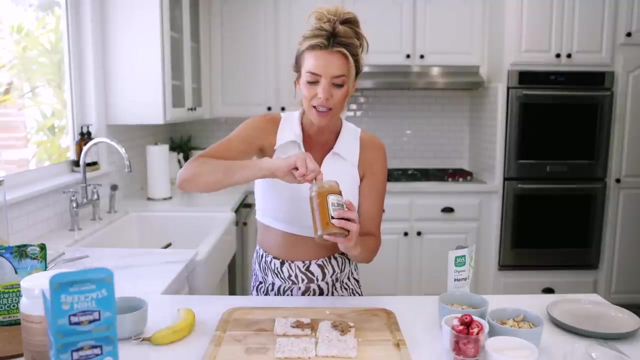 is just like the everyday without the chocolate, a little bit healthier version that you can take just for your normal day snack. so I'm going to start with those four rice cakes, again using my simple common. um, if I want to do four, then I do have to be a little bit mindful of how much nut butter I'm. 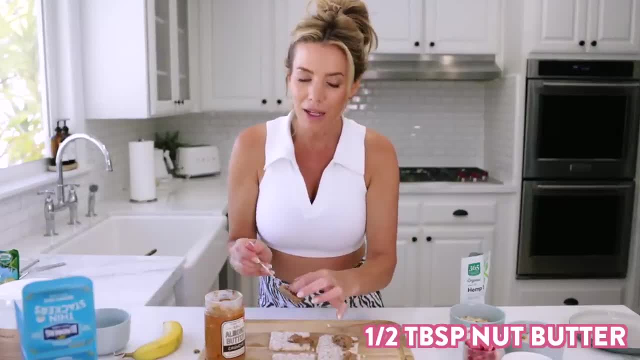 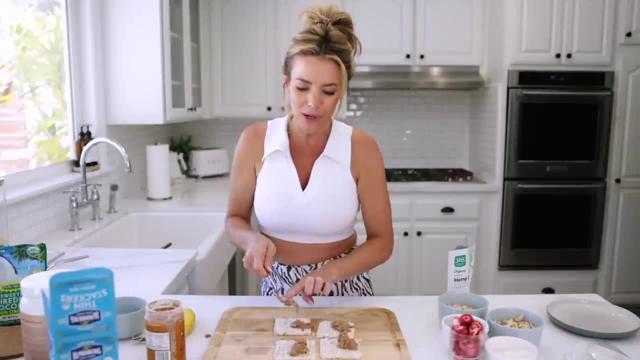 using because obviously, although it's healthy, it does have a lot of calories in those healthy fats. so, um, what is it? two tablespoons, yeah. so I'm gonna use about half a tablespoon roughly. don't come at me in the comments about like that's like a whole tablespoon. that always happens roughly on each one. 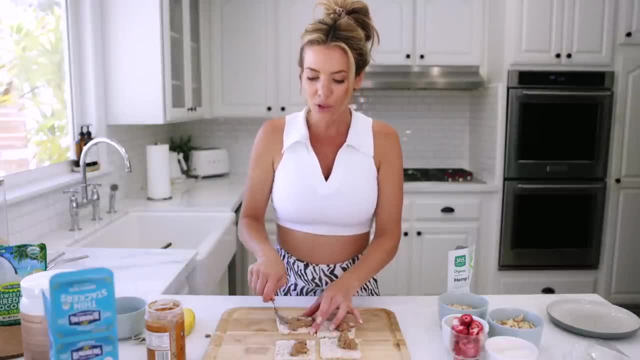 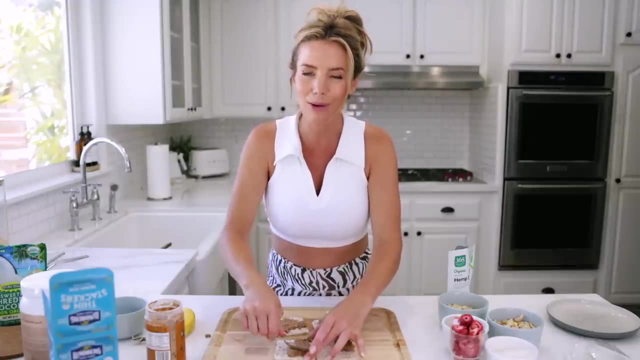 and I think that's one of the biggest things. you guys with just about half a tablespoon, that's not just like cooking or snack stuff like this. like don't stress so much about ingredients portions, like being super, super precise. we want to make it easy, so just eyeball it. you've used a tablespoon. 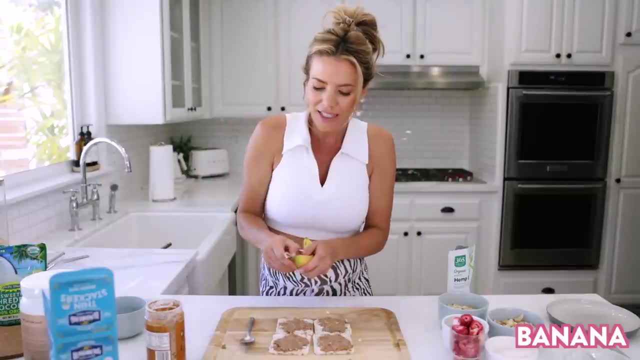 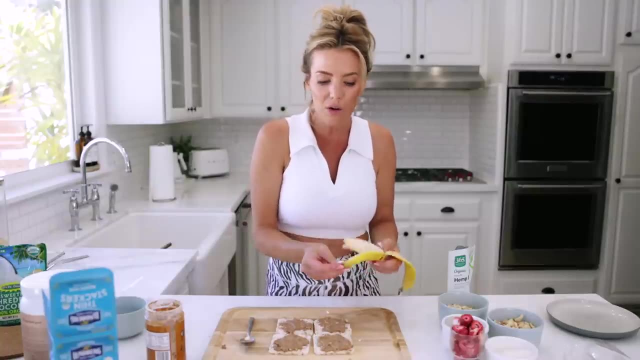 a time or two. then i'm just going to use one banana, and with this it just kind of depends on when i'm eating it. to me, i would probably have this snack before a workout. um, because there's not like a lot of protein. there's a little bit in the nuts, of course, but there's not like a ton. 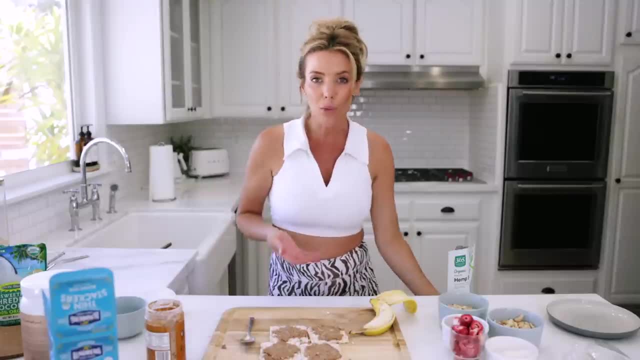 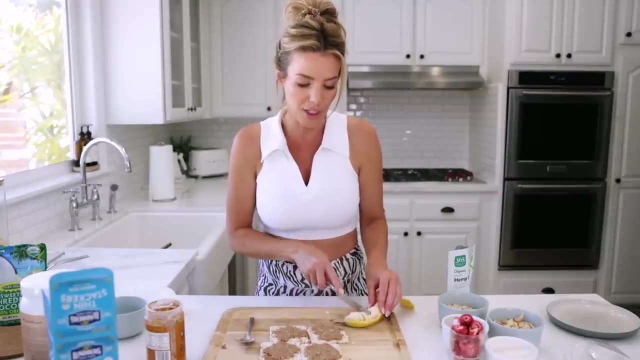 of protein, which is really important post-workout, but before a workout, the most important thing is your carbs. that's not really going to do anything for you before a workout, so i wouldn't worry too much about that, but you want to give yourself plenty of time. you don't really need those fats. 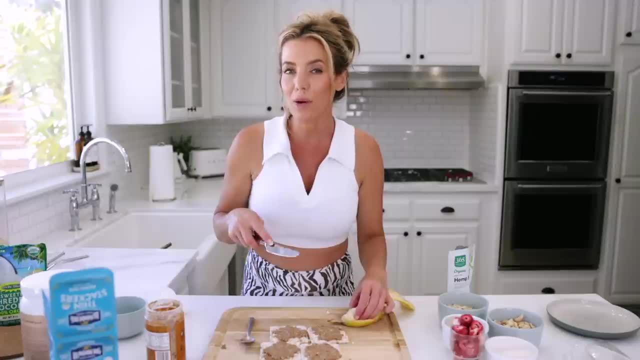 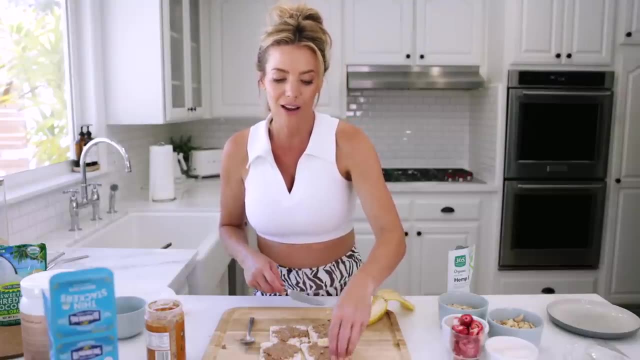 for your workout. so i wouldn't have this like within 30 minutes of my workout, but if i needed a snack about an hour to two hours prior to working out. this is going to be so great because you get all of those healthy carbs. you're going to get energy from the banana and the natural sugars in. 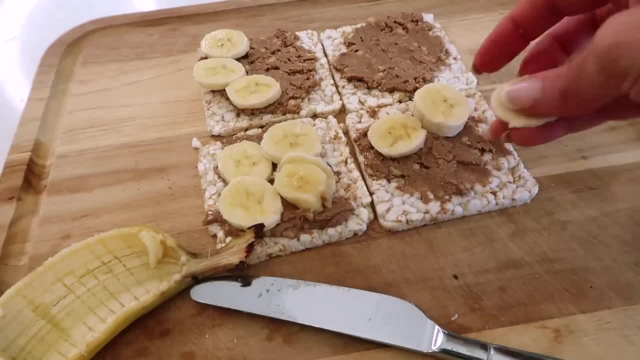 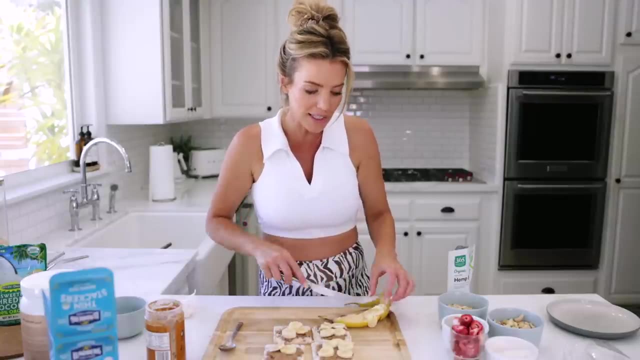 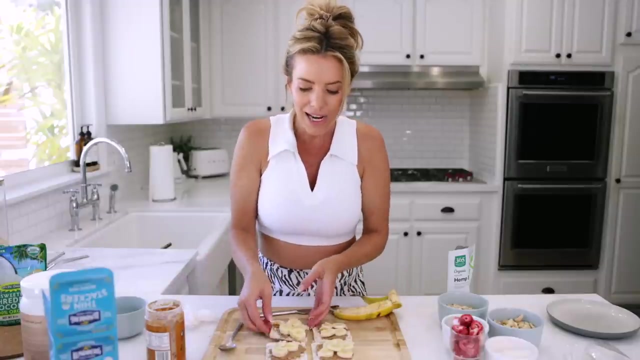 it and it will be a really good balance to fuel that. so just slice them up. you can stack these ones however you want. and then same kind of thing with this as with the more savory rice cake snack is because you have this like banana, or you have the cucumber on the other one, it just makes them. 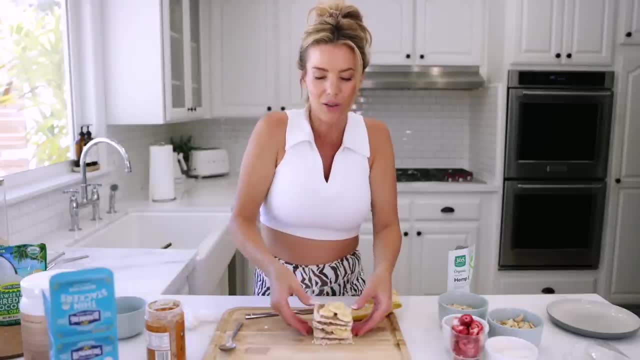 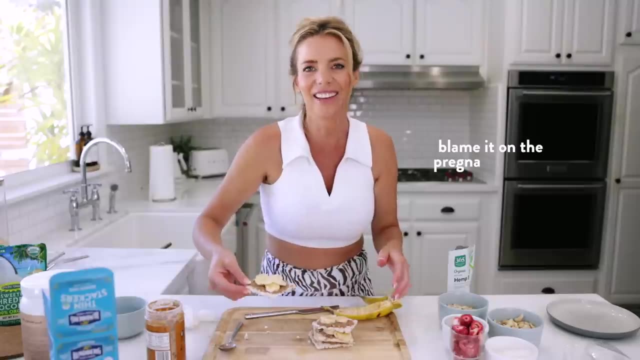 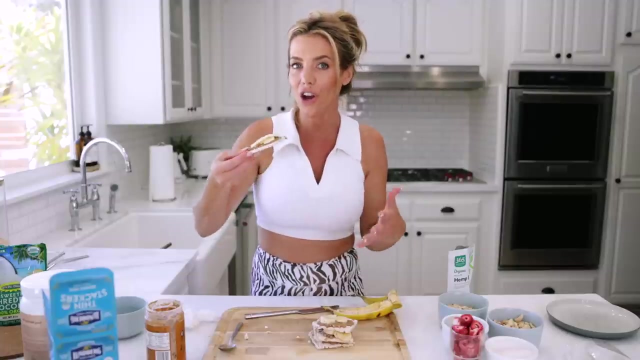 really stackable so that you can easily pack them up and take them on the go. and the great thing with these are so easy to just grab. Okay, They're so easy to grab, but they should be so easy to grab Even if you're like in the car and you need something that you can just like eat on the go in that way. 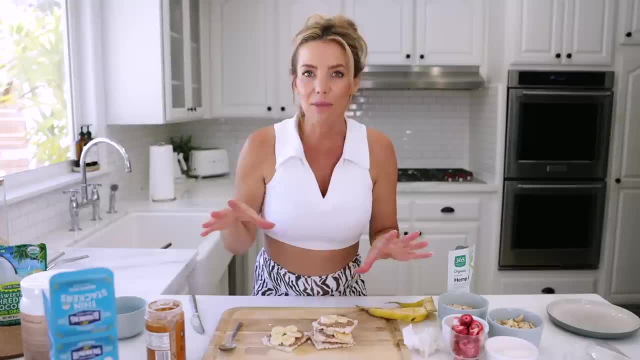 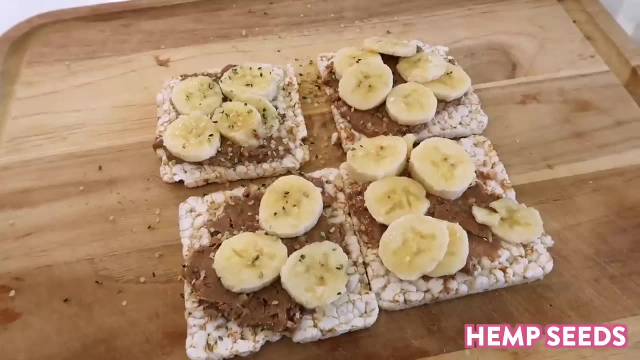 it makes for a really easy snack because everything's in like one bite. So same with all my other snacks. One thing I will say is I do like to add other things to this. So if you wanted to sprinkle some nuts on top, if you wanted to do your coconuts more hemp seed, that can. 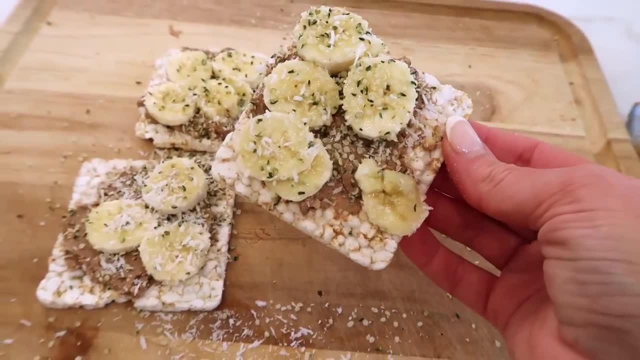 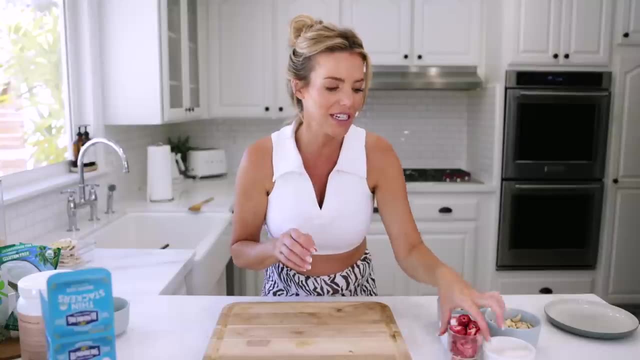 really add a little bit more flavor and more protein. which- why not? My last snack is strawberry coconut protein balls. You guys, this is my new favorite thing ever. I got these dehydrated strawberries at Trader Joe's and I didn't know what I was going to do with them. I was just like 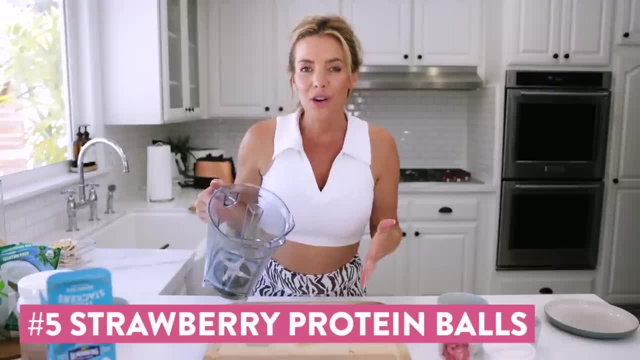 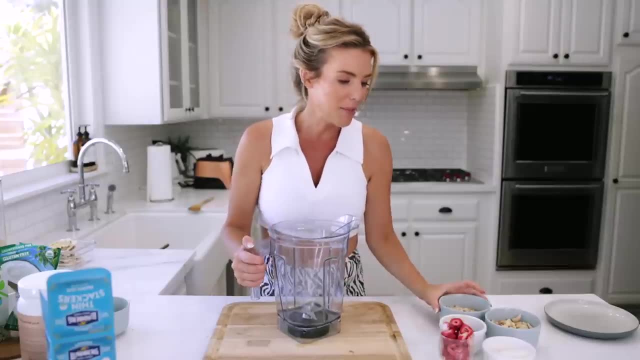 that sounds fun. And then I made this and you're welcome. I'm going to do everything in my blender. If you have a food processor, that might be a little bit easier, just because it's more shallow usually, but it works. So I'm going to start with one cup of those same oats Again. I told you a. 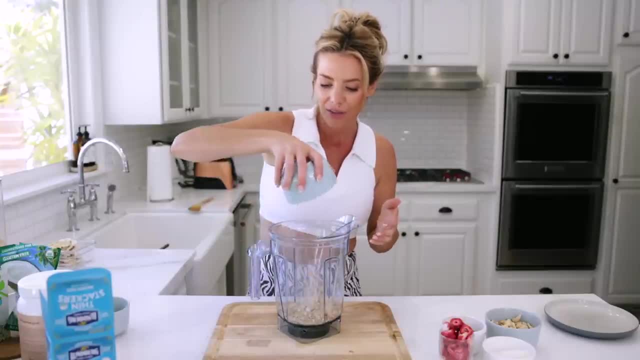 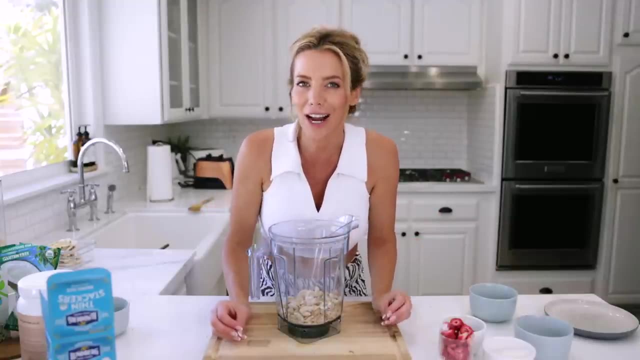 lot of ingredients that are going to be used in these, So I'm going to start with one cup of these different snacks, So one cup of those, one cup of raw cashews and, like with pretty much any recipe I ever try to give you guys, you can make swaps If you're like. I hate cashews, I only like. 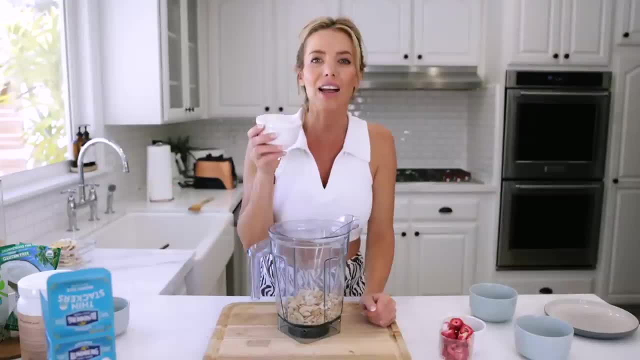 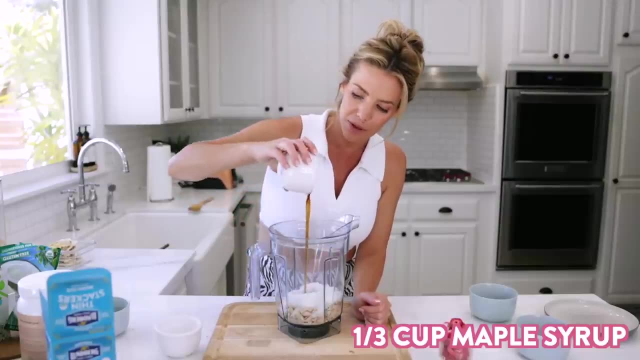 peanuts, or only like almonds or whatever. That's fine, Just swap it out. I have two thirds a cup of that shredded unsweetened coconut. We're going to add that right in. I have one third cup of that pure maple syrup. Oh, this one. I actually used a little honey too to get to the one third cup. 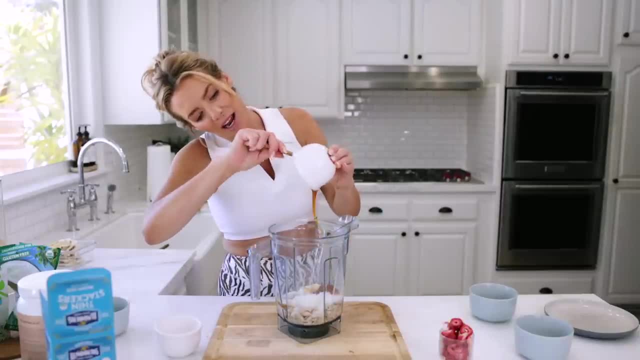 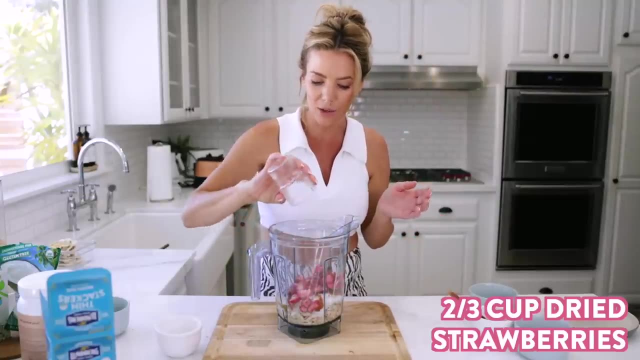 because I was out of maple syrup, A little sticky At the bottom, get that out, And then this is about two thirds a cup of the strawberries. You can add more or less, or whatever fruit you want. I like the dehydrated though, because it doesn't. 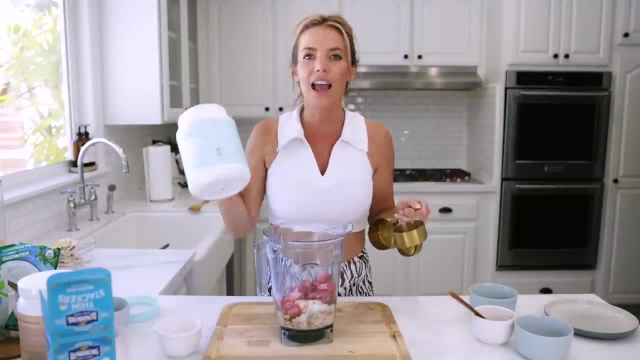 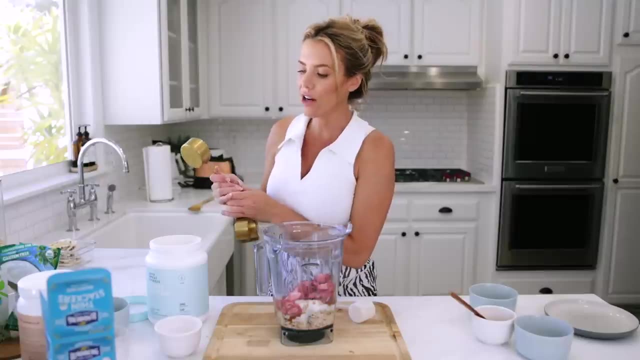 make it too soggy, Like if you were to use fresh blueberries or something. it'd be kind of weird. And then I'm going to use a half a cup of my love sweat and it's plant protein in vanilla. This is what's going to really help bind it all together and obviously give you all that protein. So all. 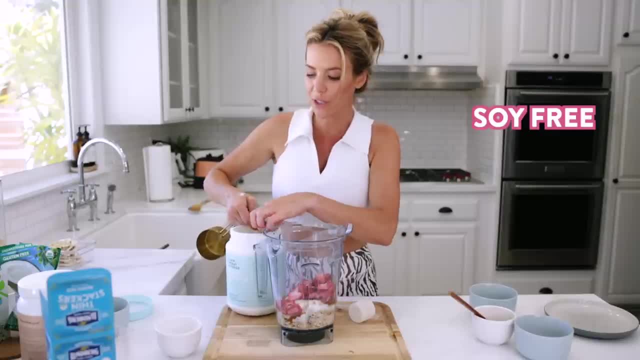 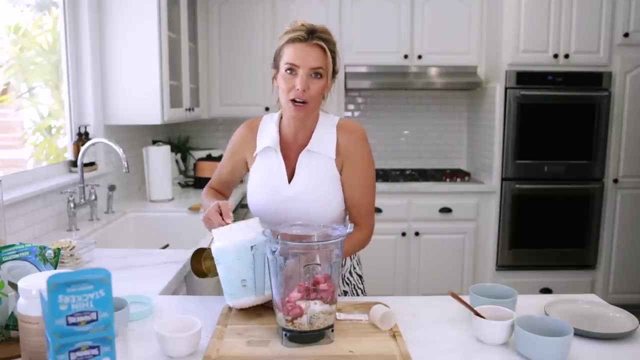 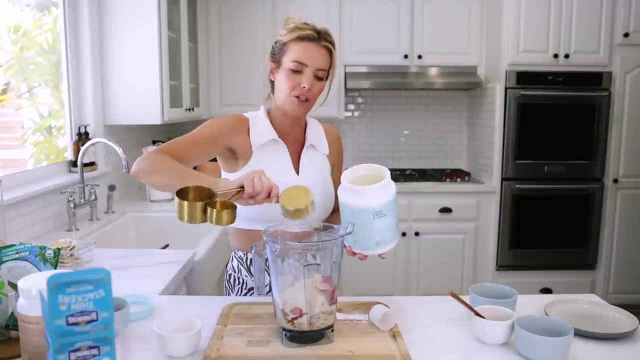 my plant proteins. just like the peanut butter, this one is gluten-free, dairy-free, soy-free, vegan, Non-GMO, organic, zero grams of sugar. I'm at like the bottom of the barrel because I use it all day, every day. So that's almost a half a cup. That should be good, And again, you can always add. 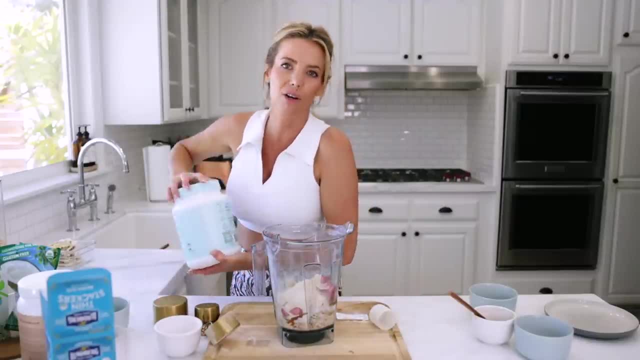 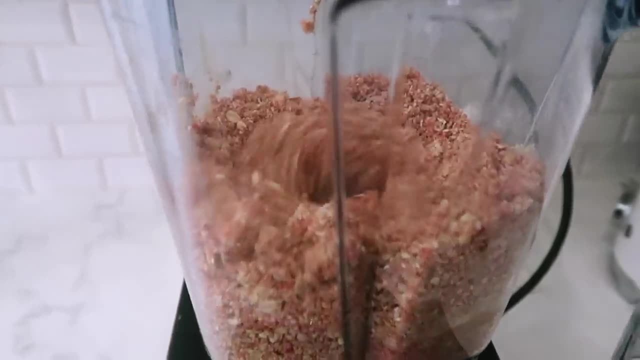 more if you need it to be like a little bit thicker, depending on how it turns out once you get blending. So once that is all ground up, you should be able to pick it up and form little tight balls. So you want to make sure the texture's right. You can always add a little bit of like. 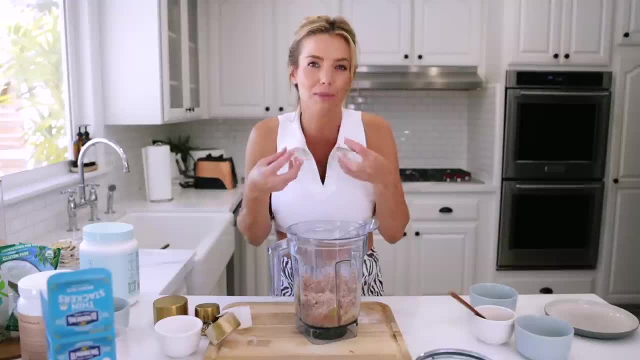 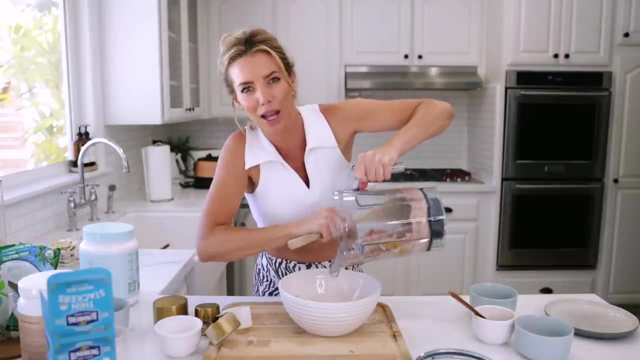 melted coconut oil if you need something to really be able to bind it a little bit better, but this one is perfect. I'm just going to transfer this into a bowl so I can get around the blade without cutting my finger. Okay, so I'm going to take that shredded coconut. 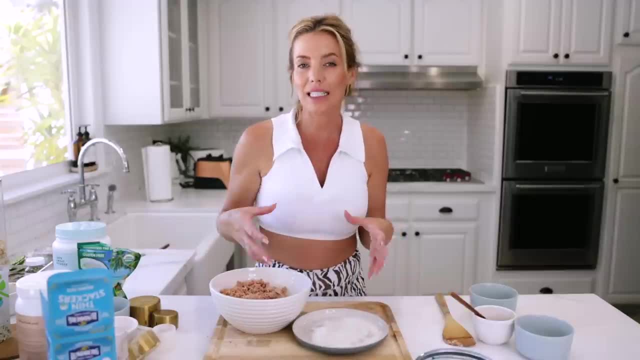 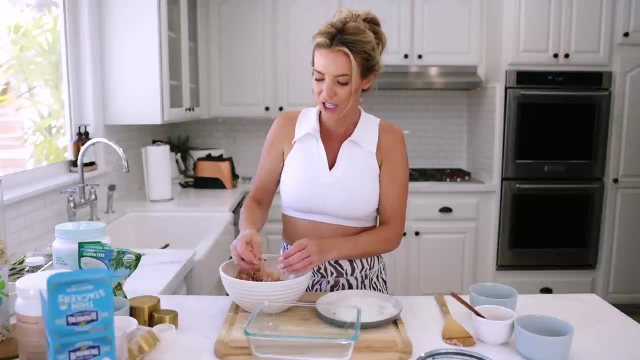 and put it on a plate and I'm going to get my container that I'm going to store these in again, because it's all about prepping snacks. You have them, not just like in the moment. So this is like a nice dough consistency. You're still going to have the crumbles, but they'll stick together. 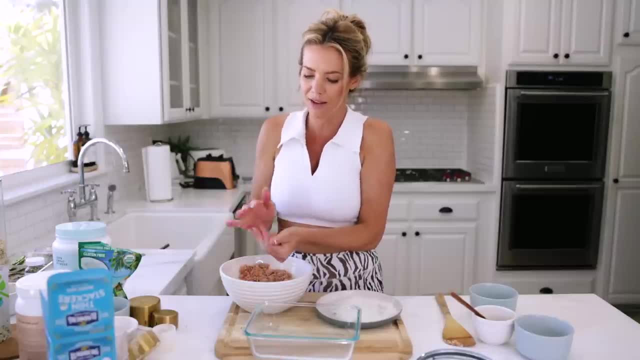 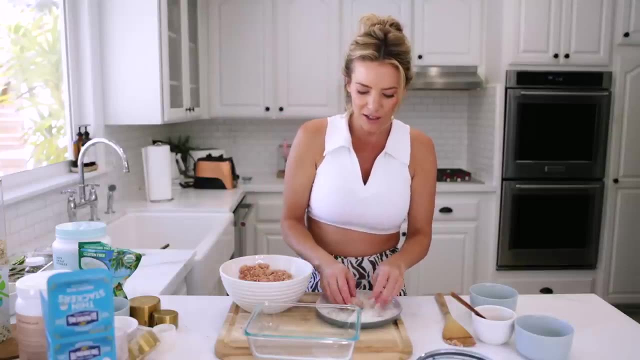 And then it's really up to you How big you want them, but I know it's like a small golf ball size, I guess. So I'll just make sure those are nice and tight, roll it in the coconut and then drop them in And you're going. 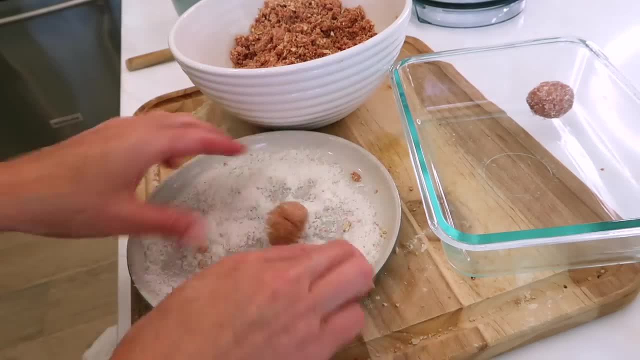 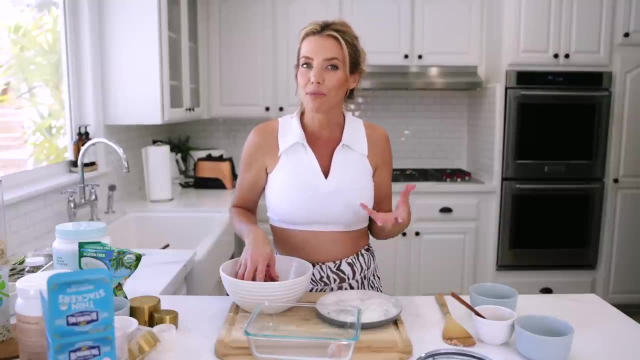 to store these in the fridge. This is also a really fun one If you have like little kids or something to have them help you, or just a husband or anyone to have help you, because it can go a lot faster. Um, this is probably the one that takes the longest to prep, but you also make. 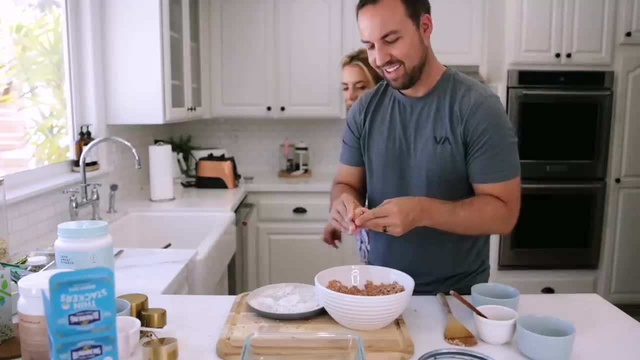 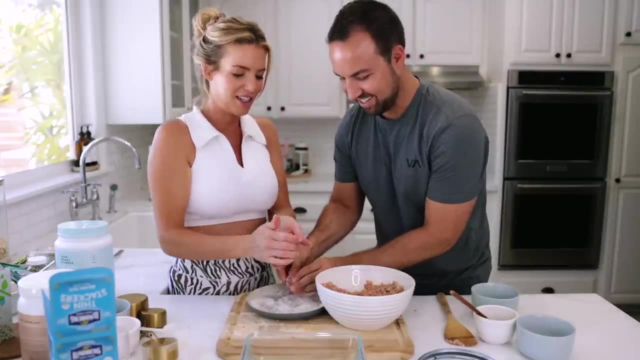 so many of them that they last you a lot longer too. Is that still your first ball? Oh, my gosh Rolling, Just squish it first. Dough balls- All right, We're in coconut. Squish it first. Yeah, yeah, yeah, We're in coconut now. Okay, That's the key. Just scoop some up and squish it.